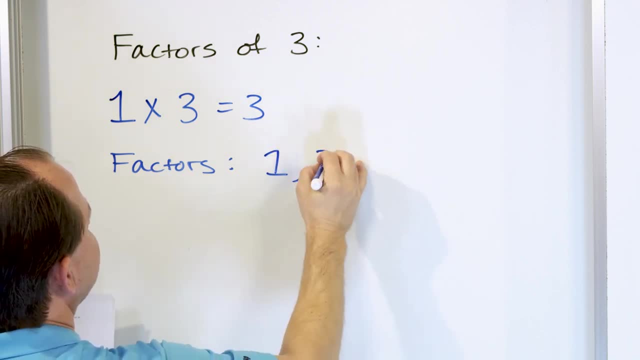 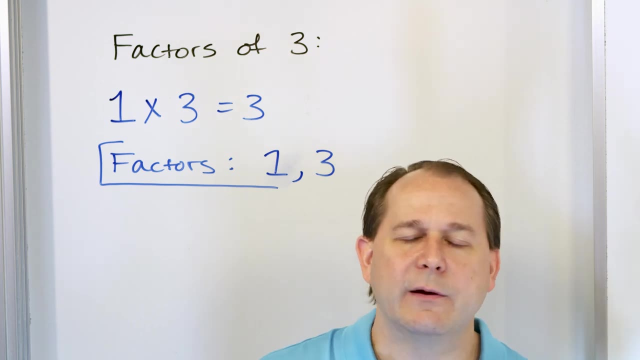 one first here. Sorry about that. We'll put the number one comma three. These are what we call the factors of the number three. One and three are the factors of three, because they are the numbers that work to multiply to give me three. all right, Now the other thing I want to do is now. 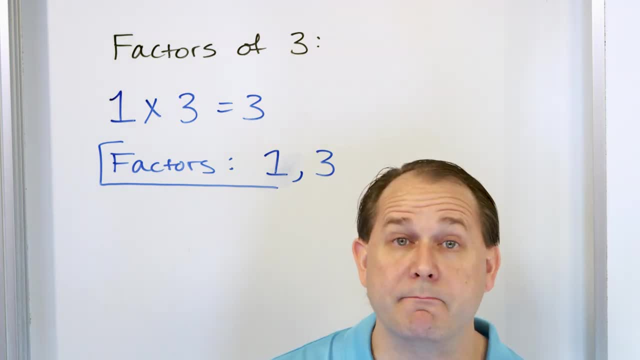 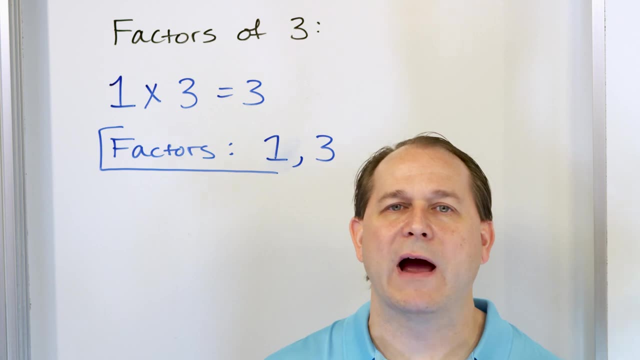 introduce the idea of a prime number and a composite number. If a number only has factors that are the number one and the number itself, then we call it a prime number. So the number three is a prime number. I'm going to write that down in a different color because that's part of 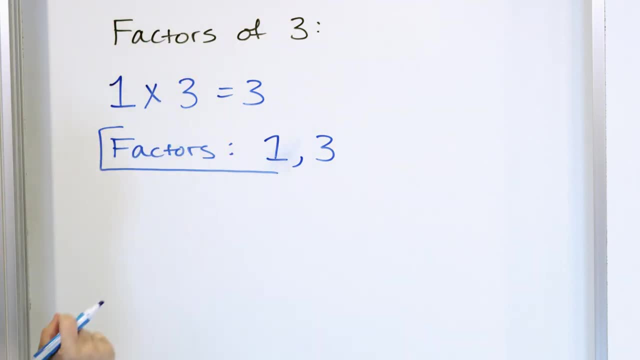 the answer. We want to write down the factors of the number and then we want to tell if the number is prime or composite. This is a prime number, So I'm going to kind of circle both of these because they're both part of the answer, Part 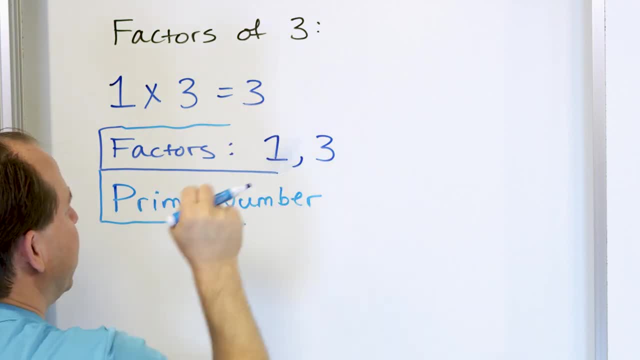 number one is: what are the factors of three? And we give the answer of one and three, because one times three is three and those are the only numbers that multiply to give me three. And then we say this is also a prime number. Three is a prime number. Why do we know three is a prime? 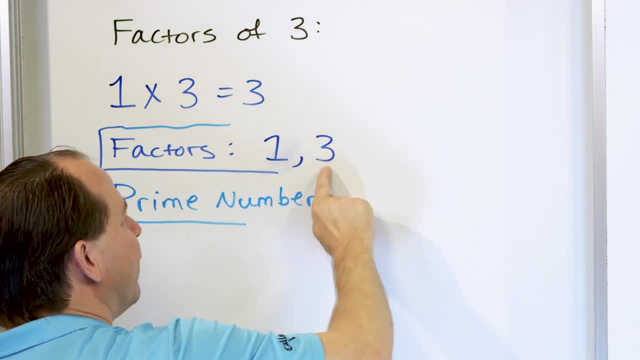 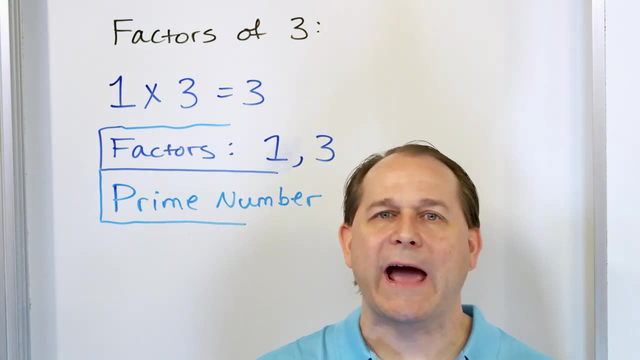 number, Because the only factors that work are the number itself, which is three, and the number one. So if I tell you, if you try to ask yourself, is the number prime, then all you have to do is say: is the number itself and the number one, and those are the only factors. it's prime, That's it. 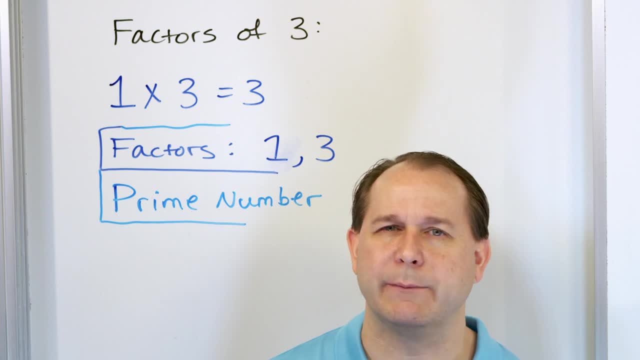 Let me give you another quick number. We'll do this example later, but I want to give you a few examples up front. I'll give you another example of a prime number: 17.. 17.. The only way you can get 17 from your multiplication tables is one times 17.. So it's prime, because only one and 17. 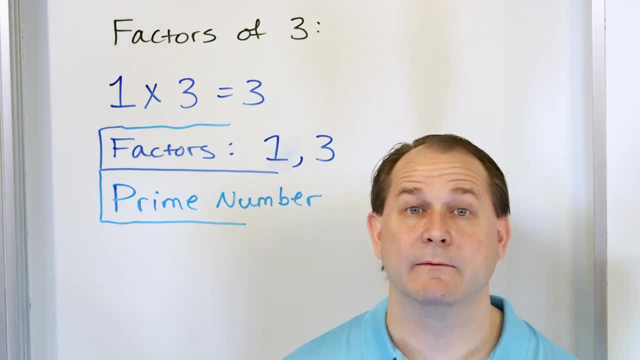 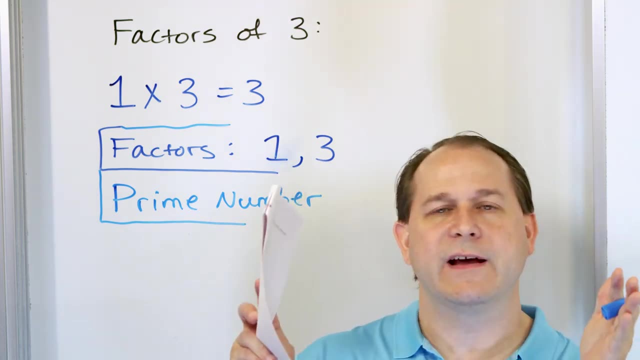 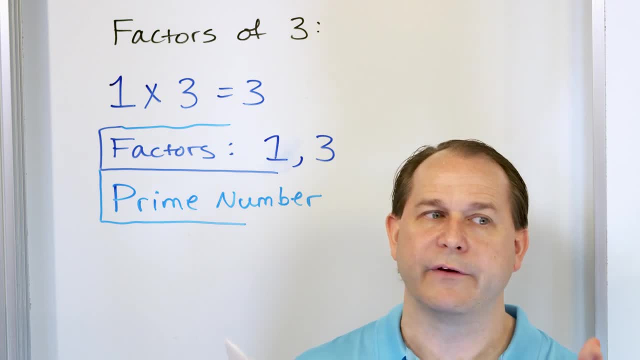 That's the only thing that works. So, because those are the only two numbers, one and the number itself, 19 in this case, then it's prime. There's other numbers: 13.. 13 is prime. See, it's all. 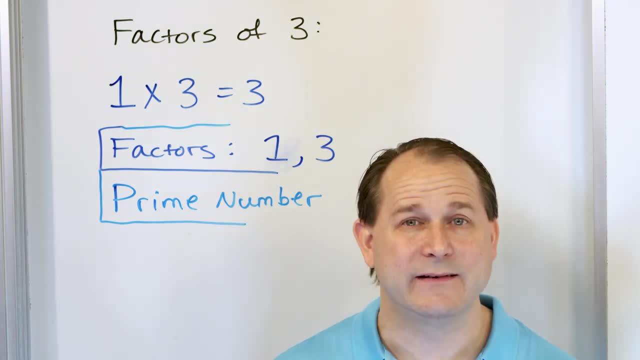 these weird oddball numbers. One times 13 is 13,, but that's it So. because those are the only two factors, one, and the number itself 13, in that case it's a prime number. So three is prime. 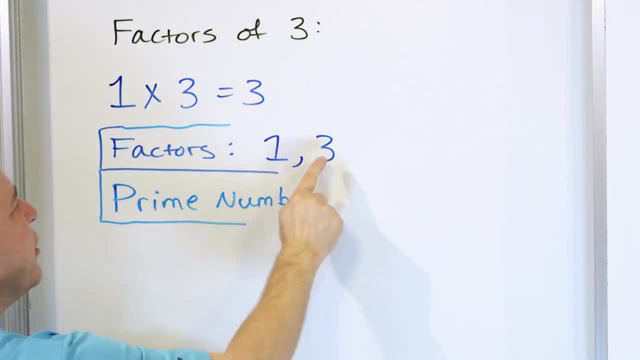 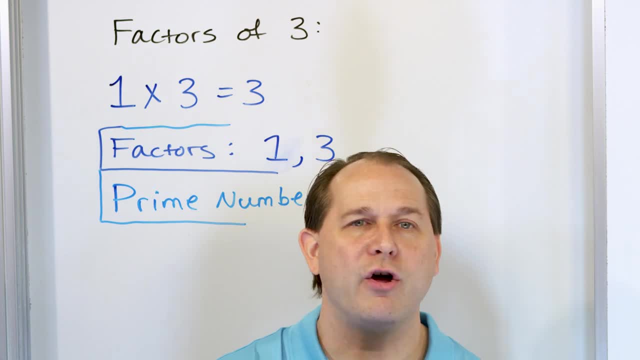 So a composite number, you might guess, is all the other numbers except for the prime numbers. Composite numbers have lots of factors. Eight is a composite number because you know two times four is eight. One times eight is eight. There's other things that multiply that give me eight. 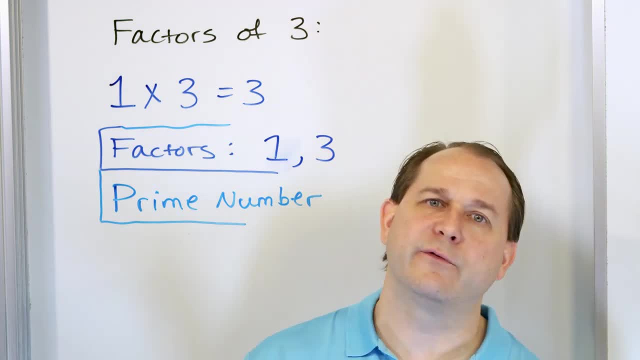 Twelve is a composite number. Why? Because six times two is twelve and one times twelve is twelve, and so on. There are other things that multiply to give me twelve. Twenty-four is a composite number. Why? Because six times four is twenty-four and one times twenty-four is twenty-four. 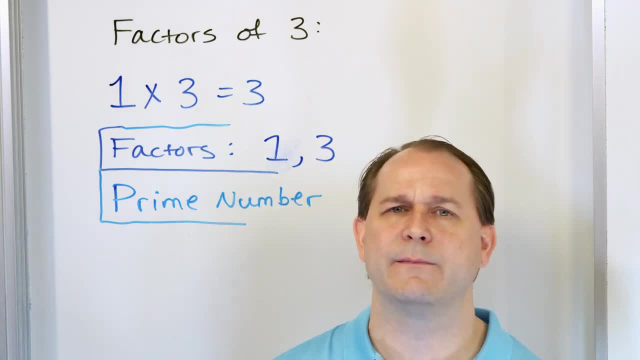 And also: eight times three is twenty-four. There's lots of things that multiply to give me twenty-four. That's a composite number. So big picture, The composite numbers are most of the numbers. Most of the numbers have lots of factors that multiply to give them. 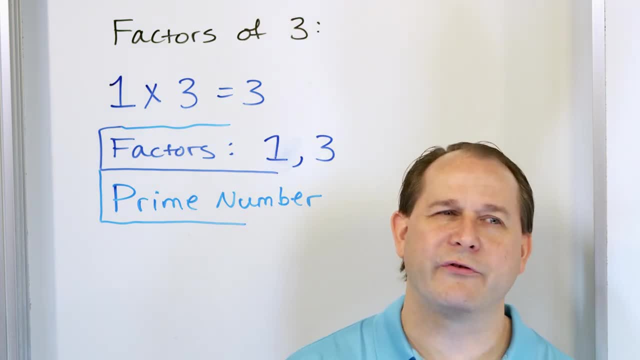 We call those composite numbers, But the special numbers are called primes. Those are the ones that only have those two numbers that multiply one times the number itself. Those are the ones that are the prime numbers with only those two factors like this. Now, the next thing I'm going to show you: 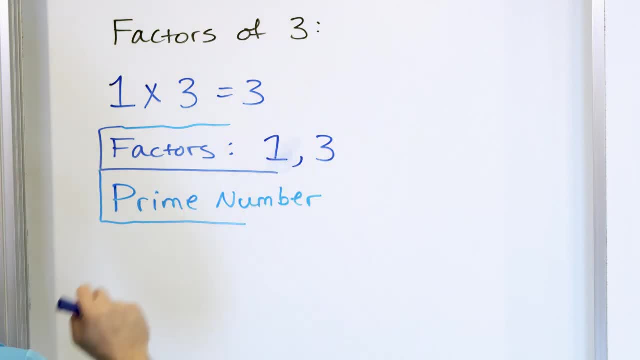 is. we thought about it in our mind how to find these factors. here I want to show you another way to find factors of numbers. It's going to be very helpful when we get to larger numbers, but I want to show you for the smaller numbers because it's really easy to understand. 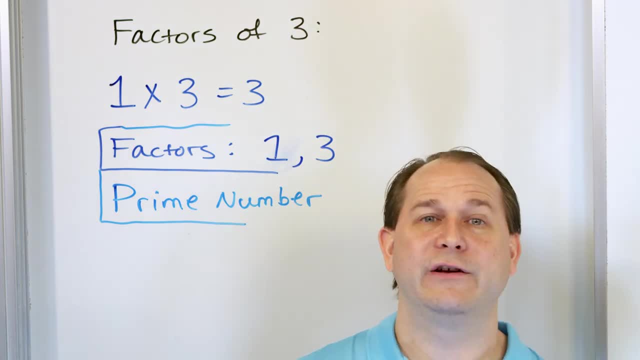 and also it's really helpful for when you get to big numbers. What if, I ask you, tell me the factors of the number eighty-four? Well then you have lots of things to think about. What times? what is eighty-four? Lots of things to think about. 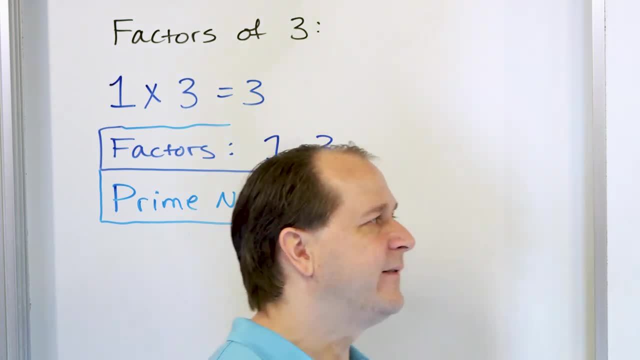 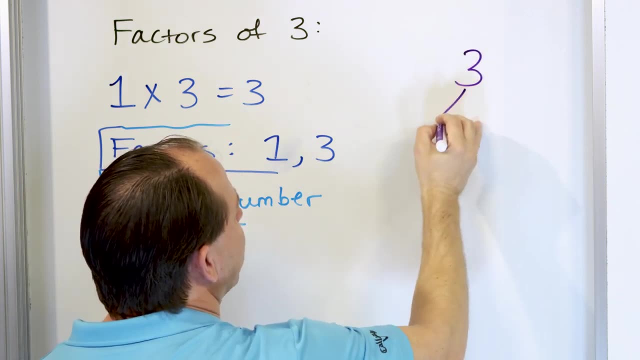 So I want to show you a great way to find all the factors. that's also very easy. So what you do is you go over here and you say I'm trying to find the factors of the number three And you build what we call a little factor tree. 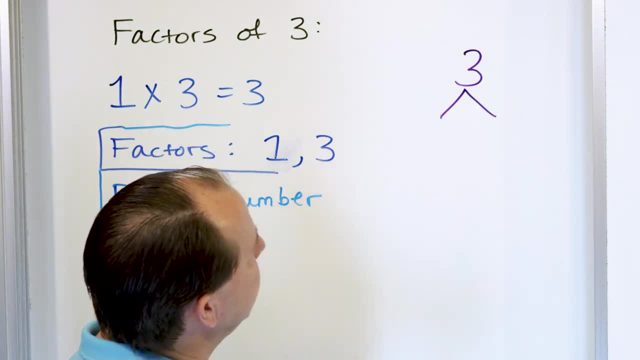 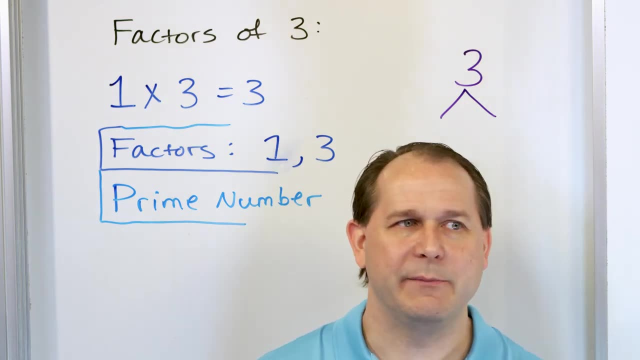 Under the number three. we try to think: what times? what is three? And you can pick anything you want, I don't care what you pick. Anything times anything is three. So in this case there's actually only one combination: One times three is three. 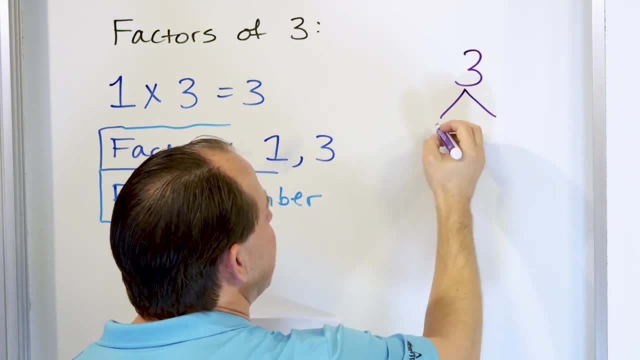 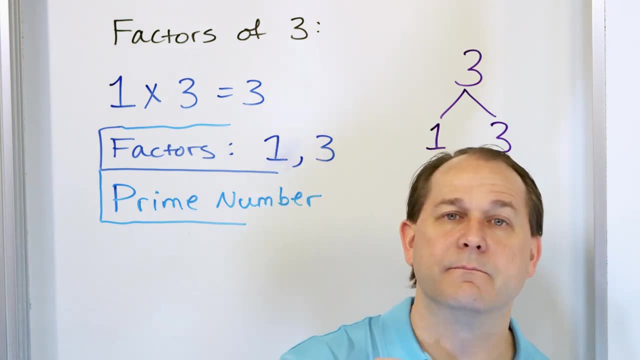 So under the tree, because we're trying to find the factors of the number three. we say one and we say three. One times three is three And up till now in your math we've been using the x as a multiplicator. 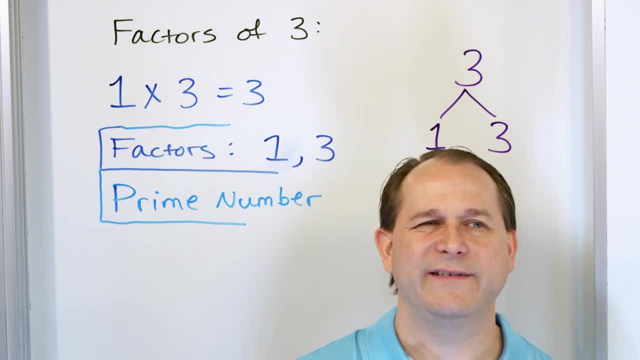 Multiplication right, Because x means multiply. But x starts to get in the way. It's a big letter And we use letters sometimes, you know, when we talked about equations earlier, So I don't want to use the letter x all the time. 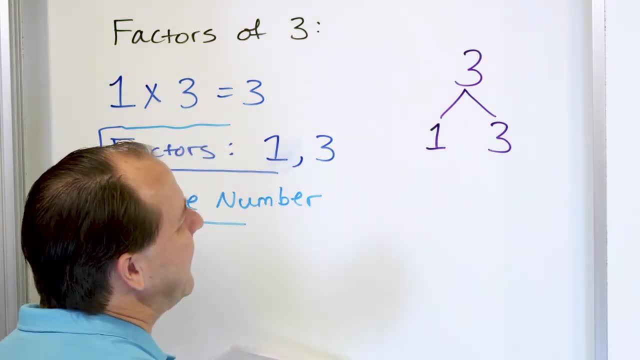 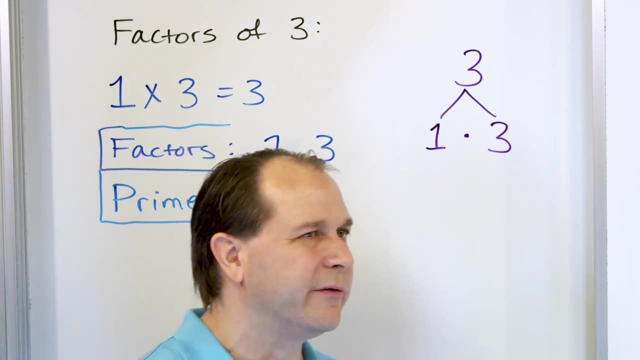 So when you're doing these factor trees, I'm going to show you another way to write that things are multiplied together. We're going to put a dot right in the middle. You need to get used to seeing that When you see a dot between two numbers or a dot between anything really. 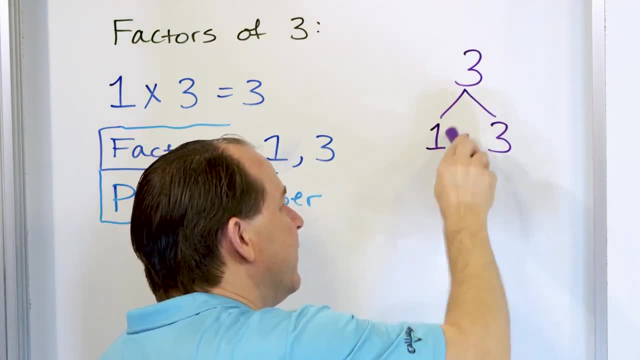 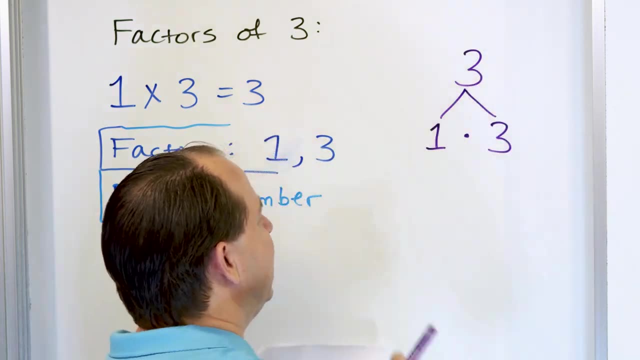 it means they're multiplied together. So I could put an x here, but it would mean one times three. But the dot means the same thing And you're going to see that more and more in math. So this means one times three is three. 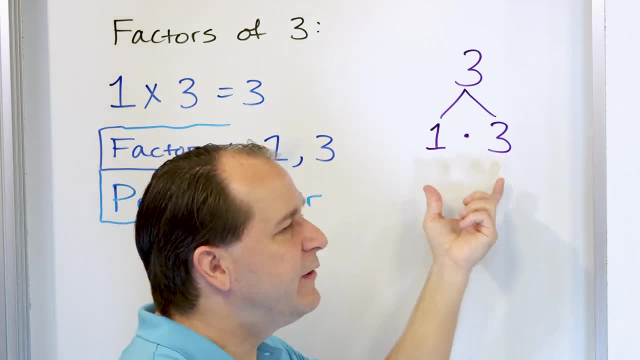 Right. So you see, the only numbers that work are these. These at the bottom of the tree are called the factors of the numbers. So we know what the answers are, because this number is so easy. But we also can make this tree. 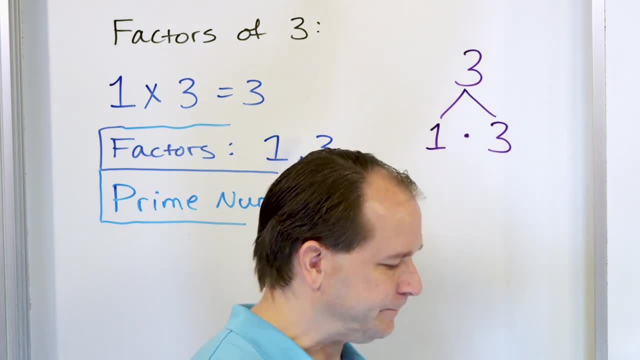 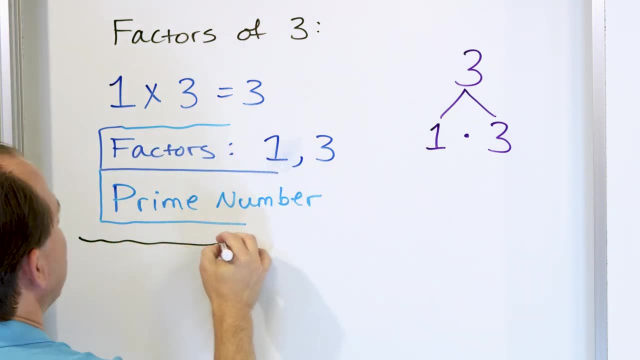 which also can help us visualize what the factors of the number are. All right, So now I think it's time for us to move back to a different problem and get some more practice with figuring out. We want to, for these problems, write down the factors of the number. 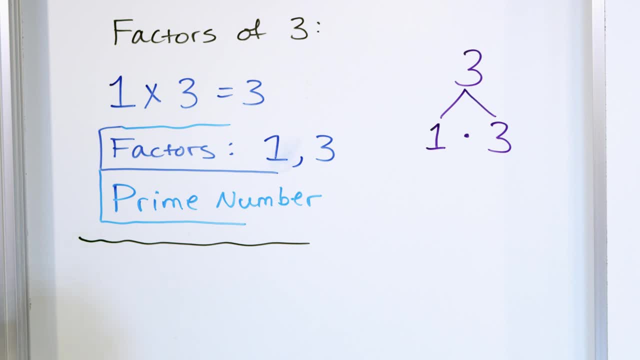 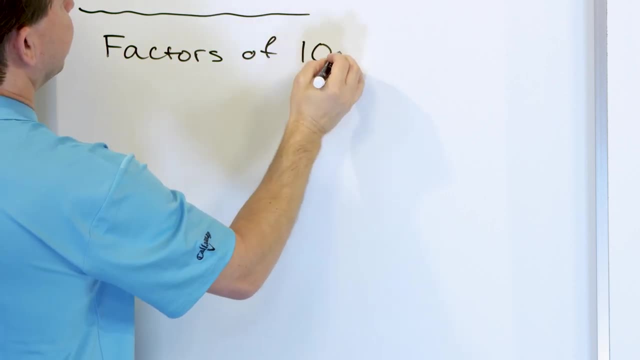 And we also want to write down: is it prime or is it composite? So let's find the factors of ten, The factors of ten First. let's do it just by thinking through our multiplication facts. Right, Well, we know that one times ten, 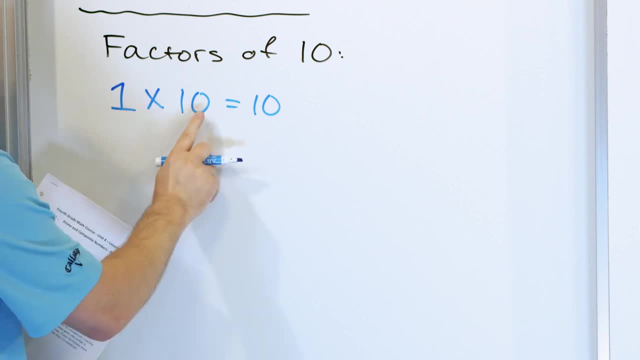 We know that that equals ten. So the number one is a factor and the number ten is a factor. We also know that. what times? what can give you ten? Think through your multiplication tables. We also know that two times five, That can also be equal to ten. 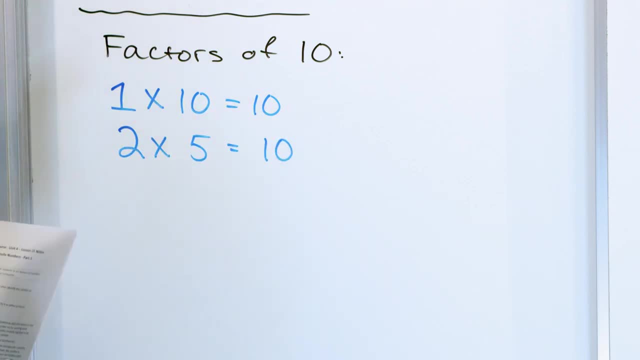 So we know that one times ten is ten, Two times five is ten, And actually that's it. So let's go ahead and write the factors down. The factors are going to be listing all these numbers here. The factors are the number one because one times ten is ten. 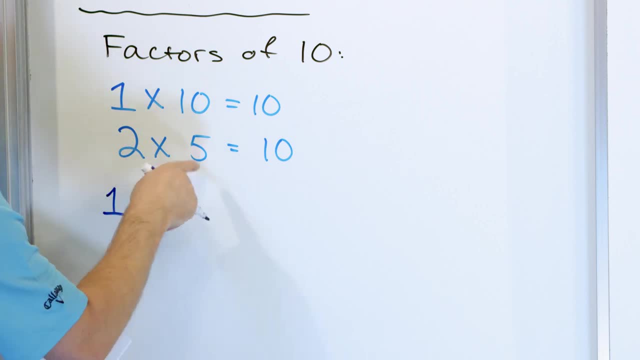 Two is a factor because two times five is ten. Right, Then we go up, up, up, up up. Then we have five. Five is a factor because, again, five times two is ten. And then ten is a factor because ten times one is ten. 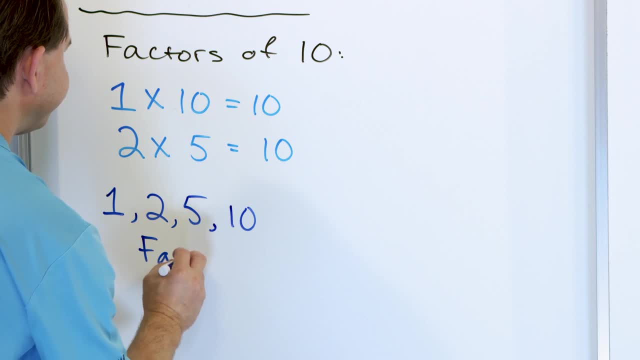 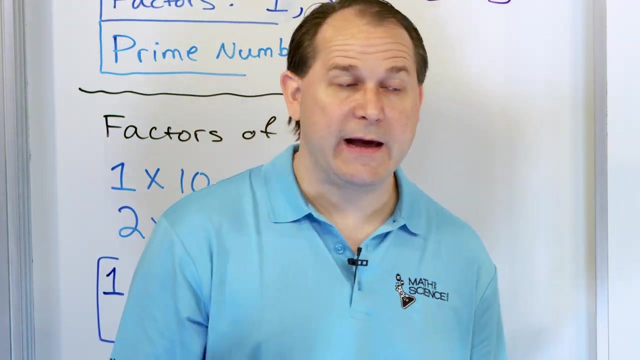 So the factors of ten- I'll put the word factors here are one and two and five and ten. Now this number, the number ten, has four factors. These are the numbers that can be multiplied together in any way throughout the listing there, to give you ten. 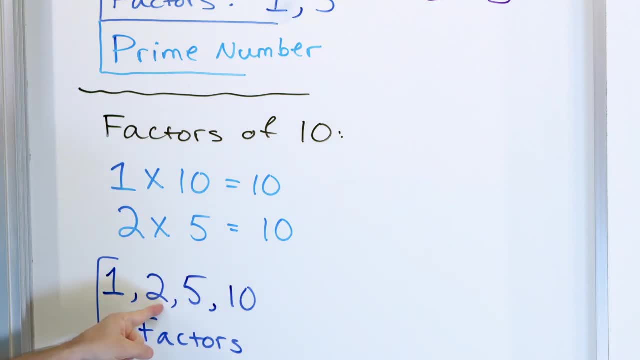 So we just go through the list. One times ten is ten: It's a factor. Two times five is ten: It's a factor. Five times two is ten: It's a factor. Ten times one is ten: It's a factor. 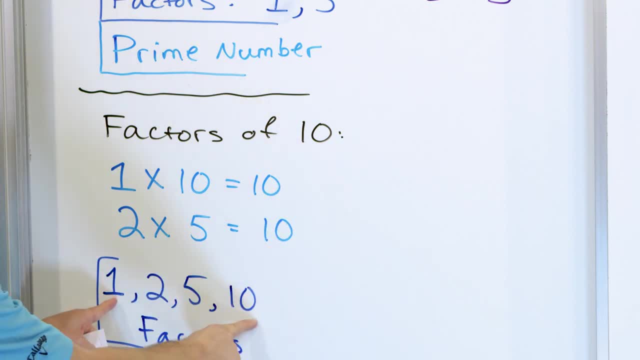 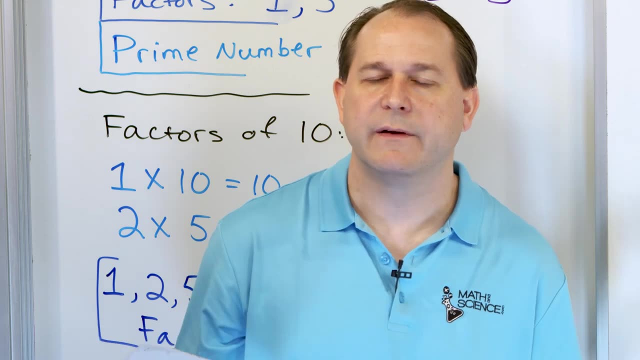 Notice that ten, which is the number itself, and one, is always a factor of any number, because any number you think of, that number times one is itself. So let's think about nine. Nine times one is nine. Let's think about twelve. 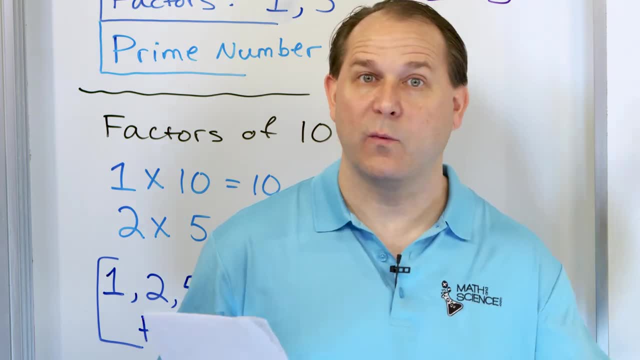 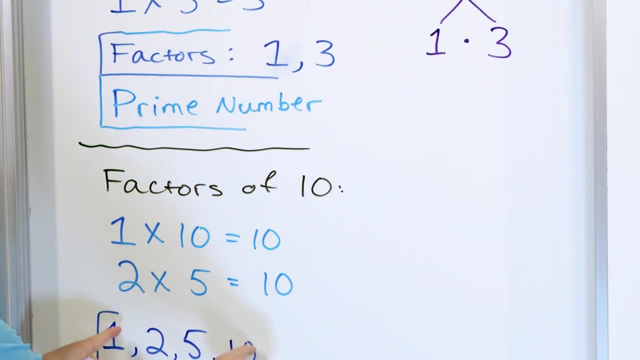 Twelve times one is twelve. Let's think about twenty-eight: Twenty-eight times one is twenty-eight. So you always have the number itself and the number one as factors, like we have shown here, and also like we have shown here, But this one's prime, because these are the only factors. 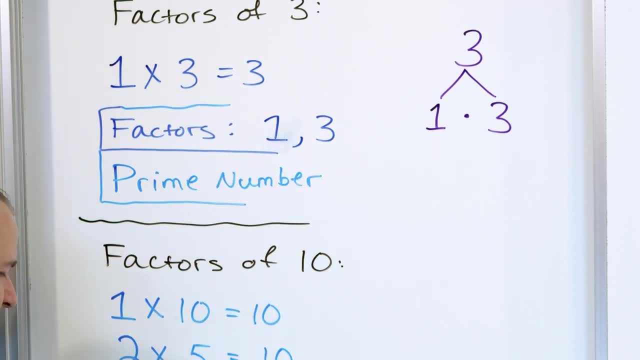 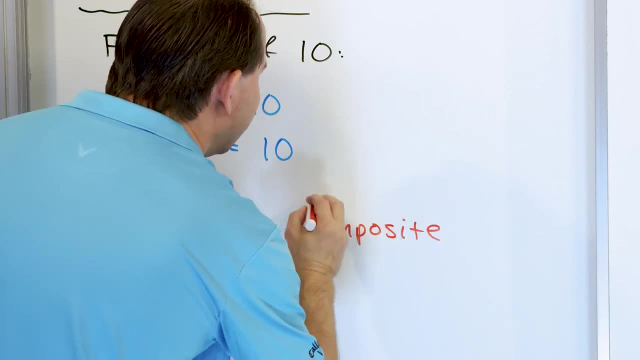 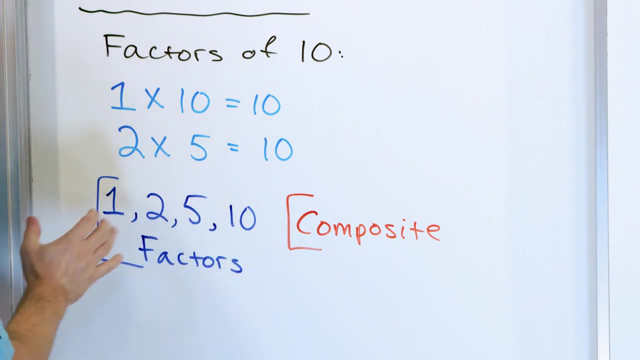 The number itself and the number one. This one is what we call composite. So we're going to write down composite because it has more factors than that. It has the ten and the one, but it also has more factors. So any time the number has more factors than the two that every number has, we call it composite. 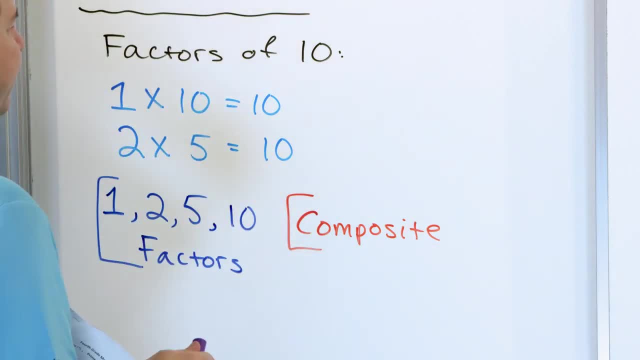 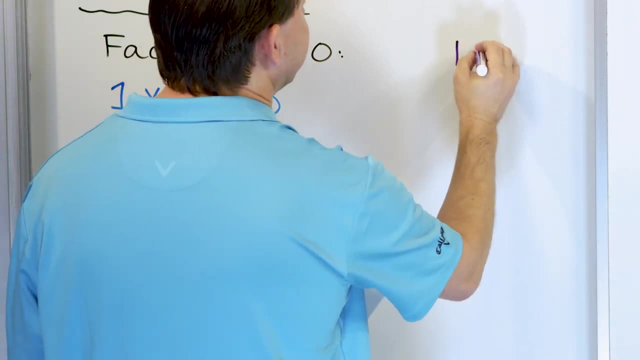 Now what I'd like to do is I'd like to show you how to figure this out with the tree method that I was going to show you. We're trying to find the factors of the number ten. So under here, I want you to tell me: anything times anything is ten. 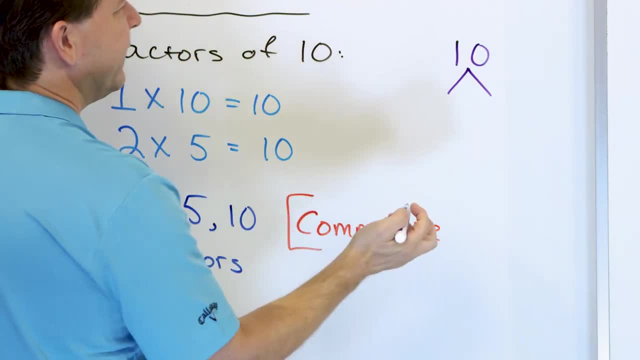 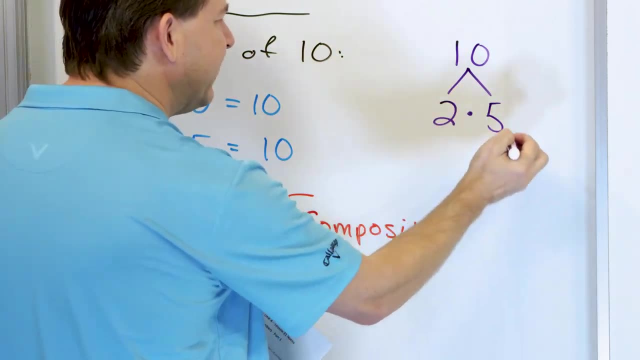 I mean, don't pick one times ten. We know those are factors. What times? what is ten? Well, two times five. Remember this: dot means multiplication. Don't let that scare you. It's just a dot. Just picture an x there. 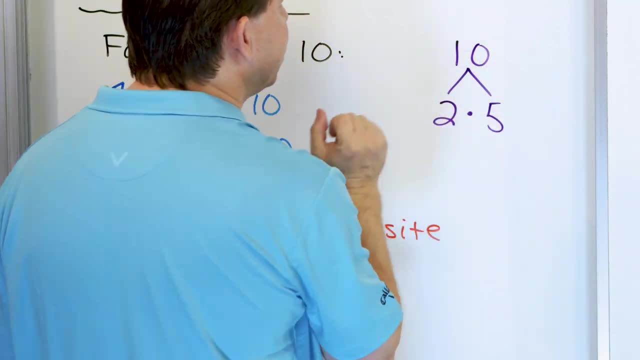 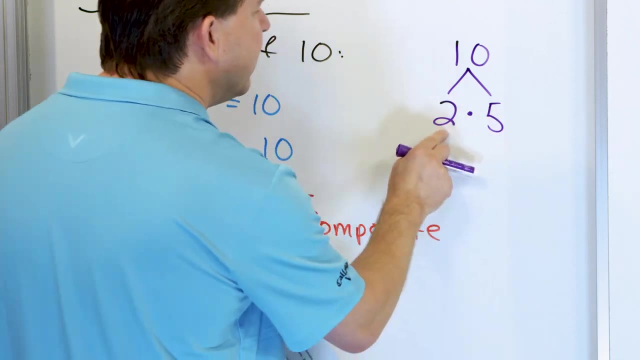 It means multiplication. So what you do is you pick the number and you pick something times. something is ten. We have two times five. Now we could make the tree go down below a four and below a five, but the only way I can write two is one times two under there. 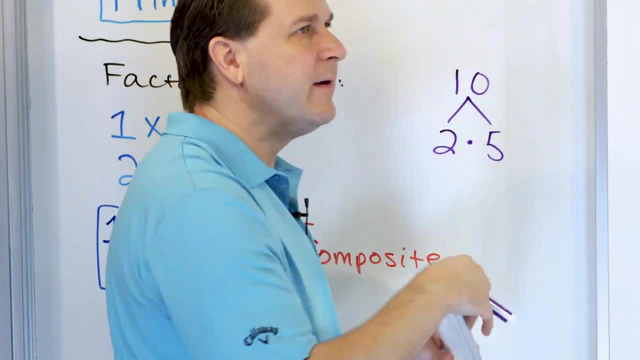 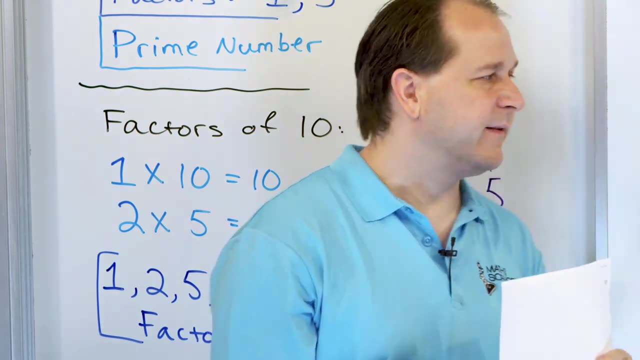 And the only way I can write five is one times five. So when you get the tree down to the point where the only thing at the bottom is just- I can't really make the tree any deeper really, because the ones at the bottom are just one times two and one times five- then I can just stop. 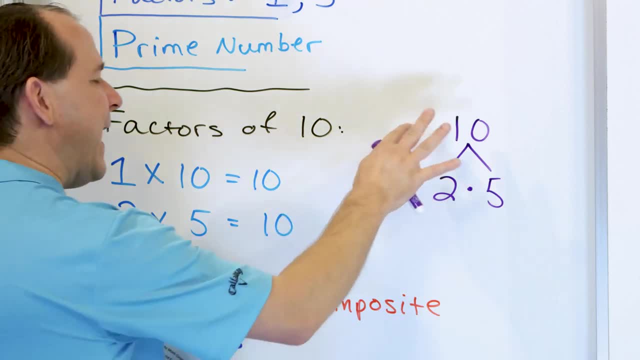 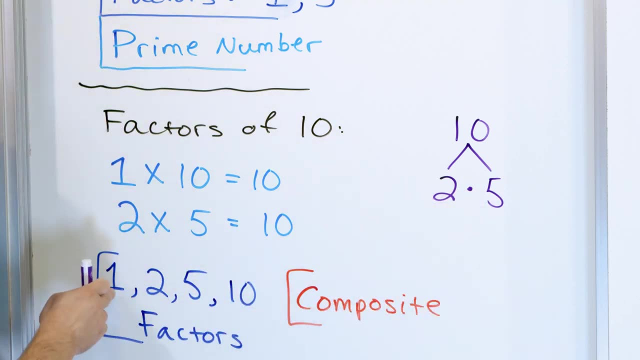 And I can read the factors right off the tree. So the factors are read right off the tree like this: I know that two is a factor, I know that five is a factor, And then for every number, number one and the number itself is also a factor. 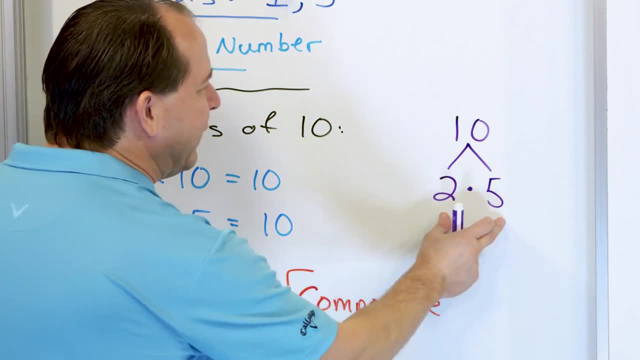 So I always put those in the list. But all the other numbers, I can just read them right off the tree. Now you might say: why is he doing this tree business? It's so easy to think of this. Well, it's easy when the number is ten. 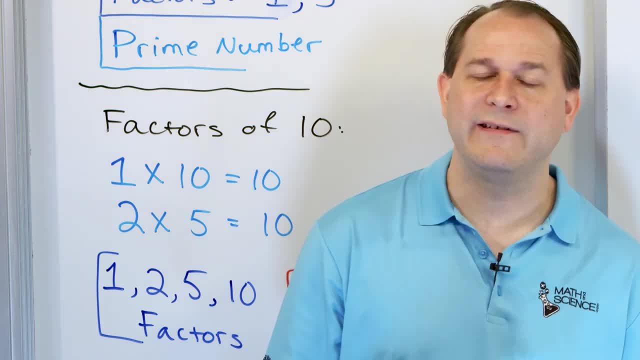 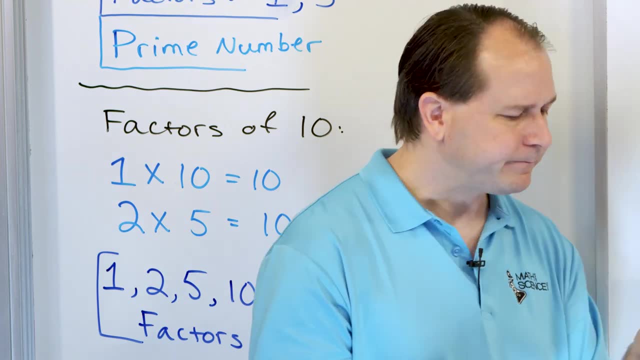 But if I give you the number ninety-six, it might be a little harder to tell me all the factors. So we're going to use these trees for the bigger numbers. I'm also going to show you here for the smaller numbers as well. 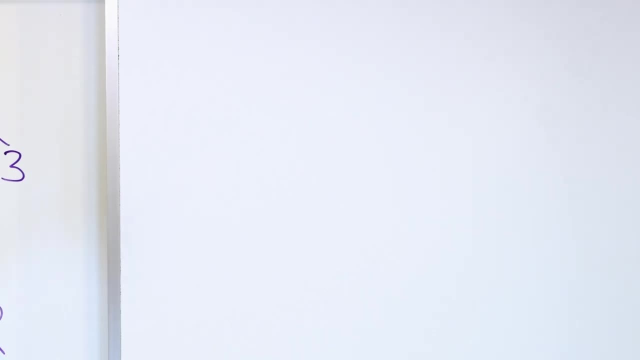 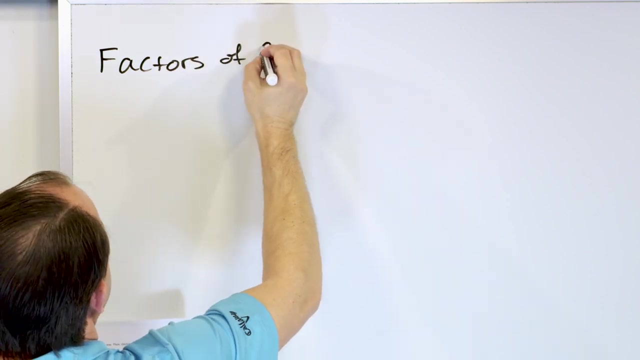 So, now that we know the basic idea, we're going to speed things up just a little bit. So what I want to find is the factors of the number nine. We're going to find the factors of the number nine, So we have to think through what times. what is nine? 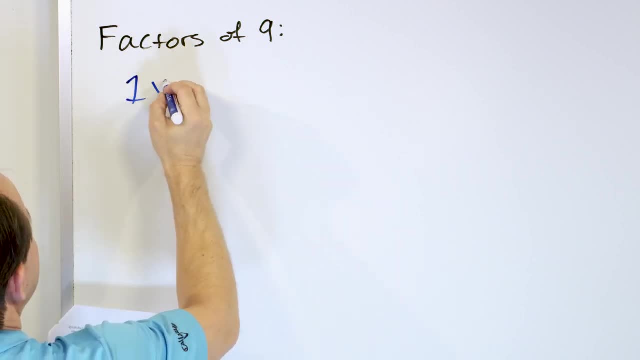 What times? what is nine? Well, I know that of course, one times nine is nine, right, Of course, I have two times, that doesn't work, is nine. But I get to three and I say: oh, I remember, three times three that's equal to nine. 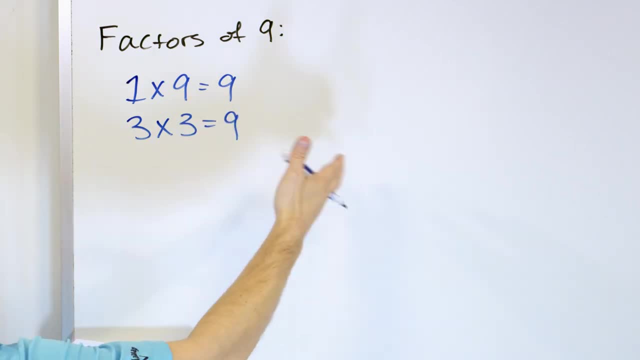 Okay, And then I keep going. Four times, nothing is nine. Five times nothing is nine. Six times nothing is nine. Seven, eight, none of those times anything is nine. So really, these are all the factors. So the factors of the number nine are: 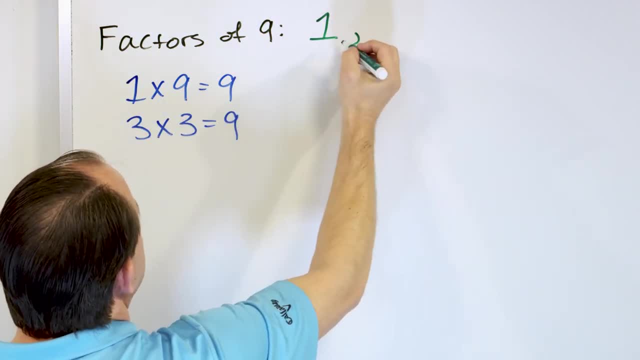 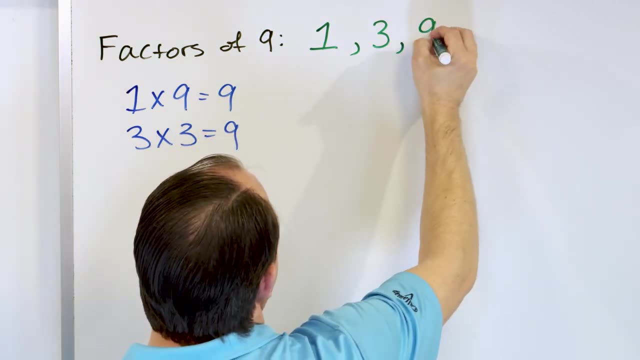 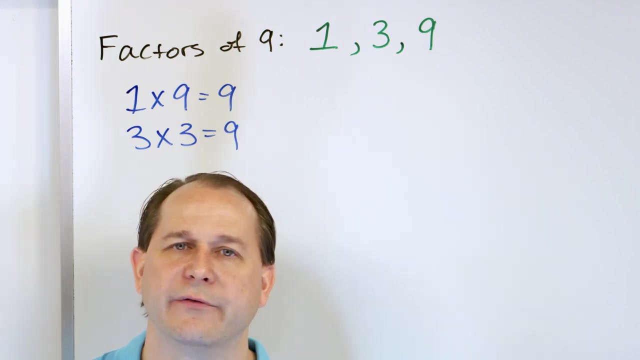 One because one times nine is nine. Three because three times nine is nine. I'm sorry, three times three is nine And then nine because nine times one is nine. Now I have three repeated here. When you're just listing the factors, you don't have to list all the repeated numbers. 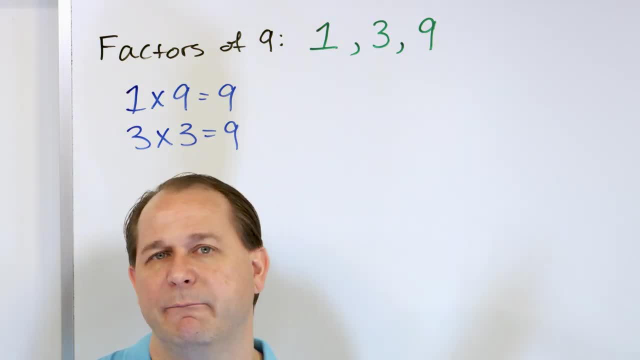 We're just trying to find the numbers that can be multiplied together to give me nine. So if I have duplicates here, I don't need to count them. So the factors of the number nine are one, three and nine. All right. 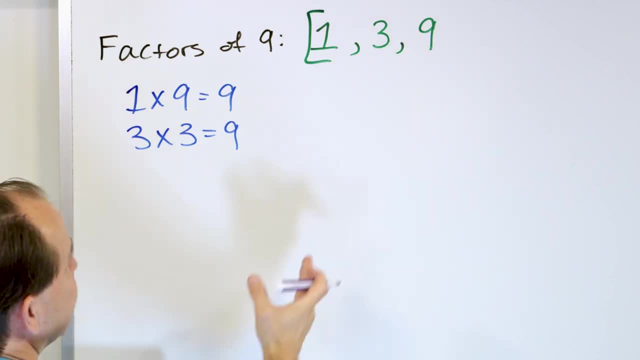 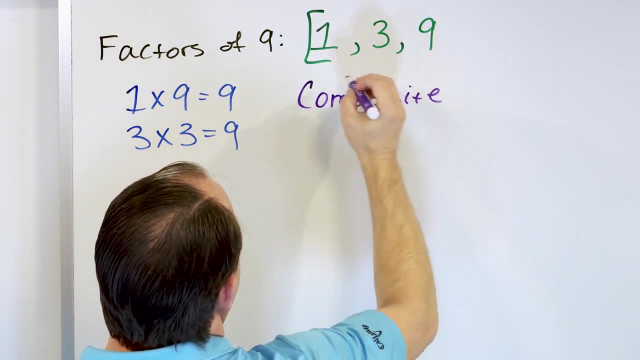 Now let me ask you a question: Is this number prime or composite? Well, it looks like it has more than two factors, so it has to be composite. So I'll put composite here, Right See, the number nine has always as a factor the number itself and the number one. 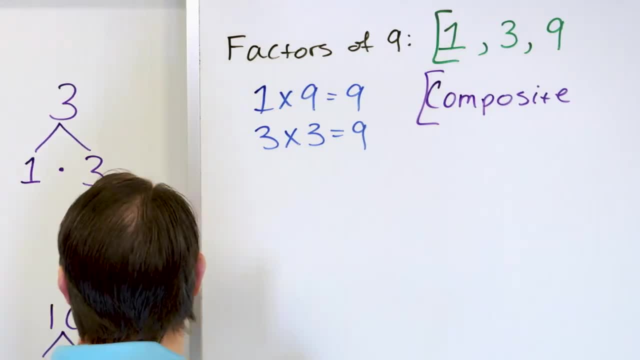 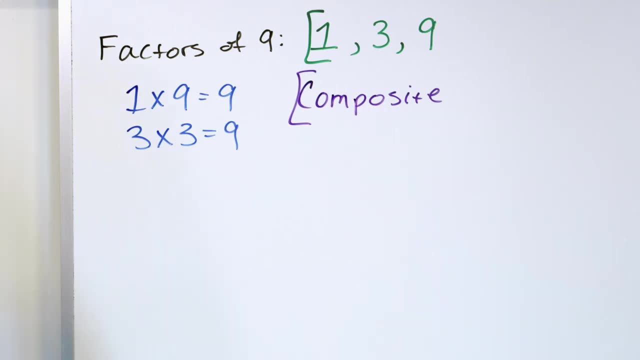 But it also has this factor. so it can't be a prime number Because, remember, prime numbers only have these two factors: the number itself and the number one. Now let's go off to the side and let's do our little tree thing. 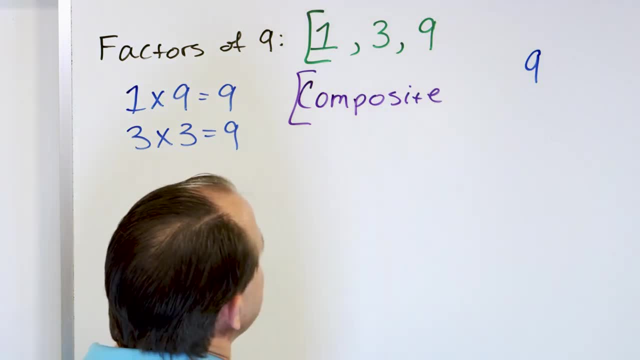 We're trying to find the factors of the number nine, All right, So what do I do? I'm thinking: what times? what is nine? Okay, So I'll build a little tree here And I remember: three times three is nine. 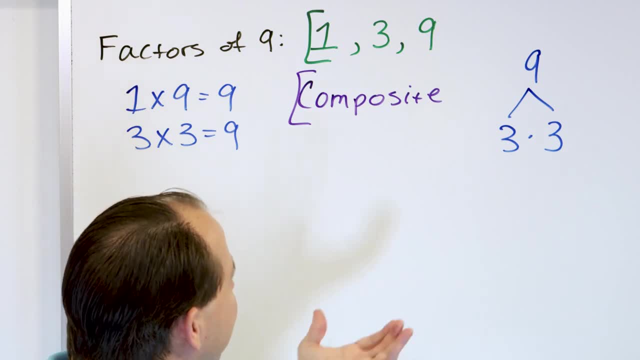 So I'll put a three times a three here. Three times three is nine. So when I read the factors off this tree I just see that there is a three here, And I make sure I put three in my list of factors. 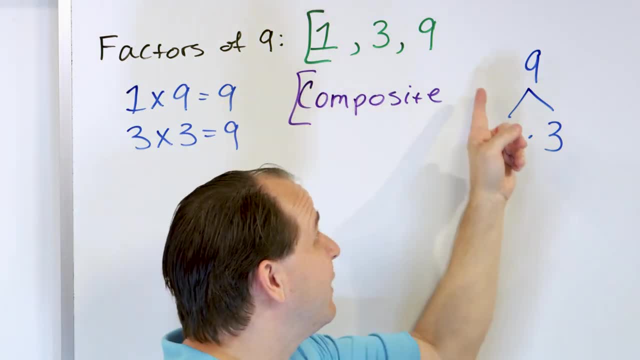 But in my list of factors I always have the number one and I always have the number itself. So those I don't really read them off the tree. The tree is used to tell me all the other factors. I know that one is a factor of nine. 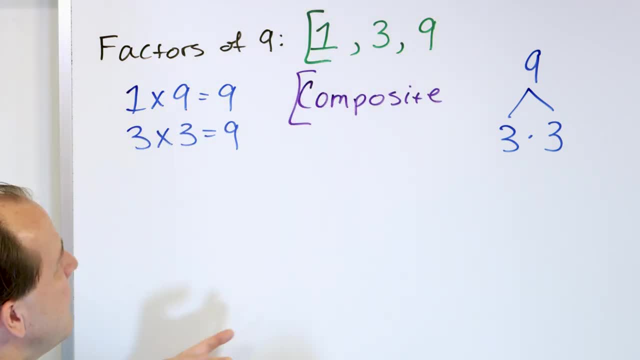 And nine is a factor of nine, Because one times nine is nine. The tree helps me find out any other factors. So this is a composite number And that is the final answer. All right, Let's take a look at the next problem. 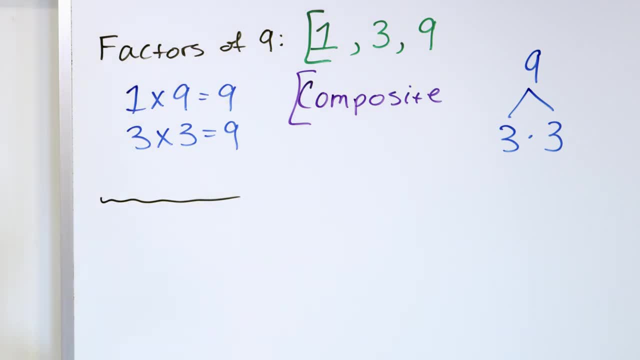 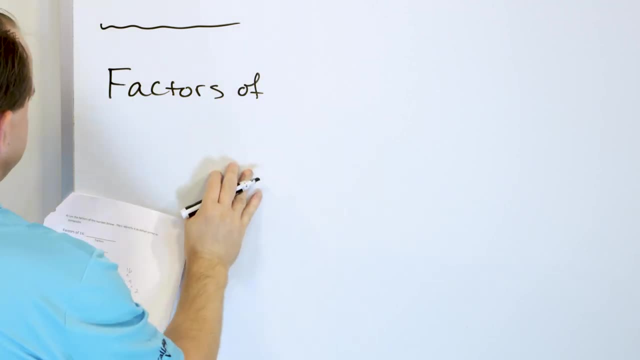 Let's find- Actually, we've already done that one. Let's skip to the next one here. Let's find, Let's do another one that's a little bit larger- Factors of Factors of the number 16.. All right, 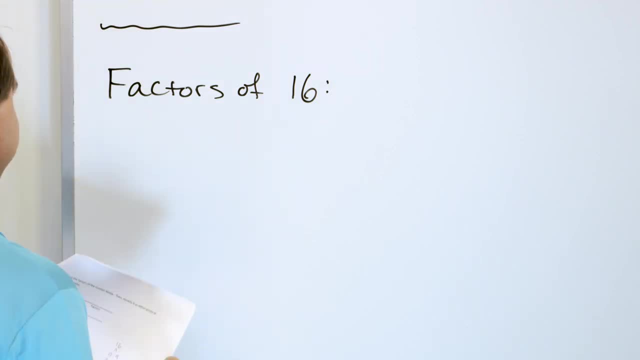 So what we have to do is just think about what multiplies together To give us 16.. Well, we all know that, of course, one times 16. That's 16. That's for every number. So the number one and 16 are factors. 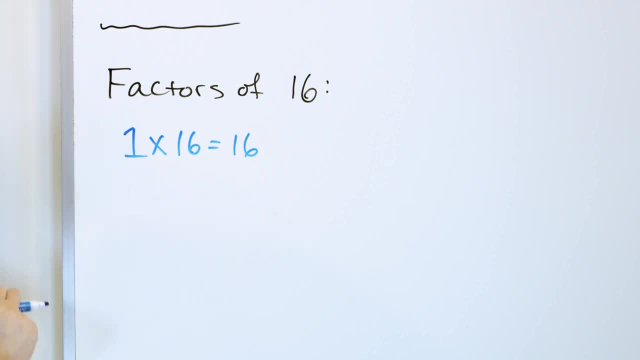 If these were the only factors- one and 16, it would be a prime number. But we know that we have more factors, So let's move up. Let's move up to two. Two times what is 16?? Two times eight is 16.. 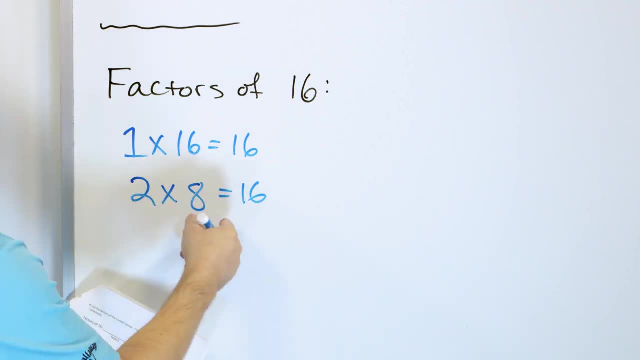 So two and eight are also factors. Let's go up Three times nothing works to make 16.. But when I get to the number four, I remember that four times four is also 16. So four is a factor as well. 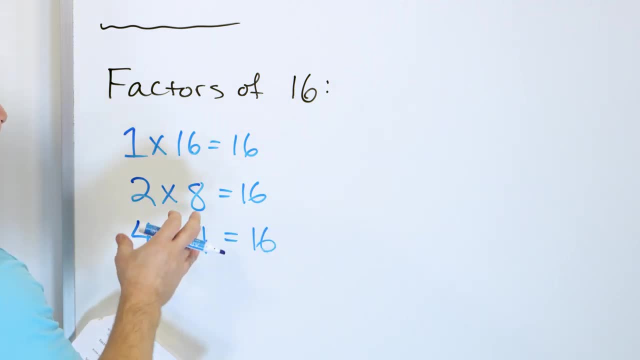 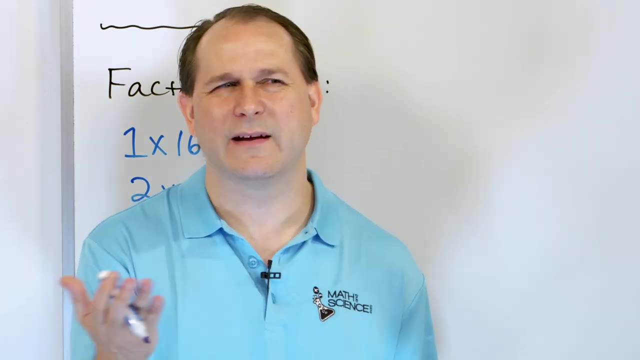 Then I go to five. That doesn't multiply, to give me 16.. Six doesn't multiply. You might think six works, but six times nothing, it doesn't really work to give you 16.. Then you go to seven. Seven times nothing is 16.. 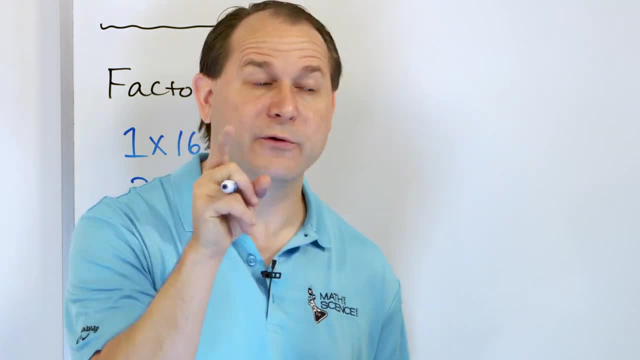 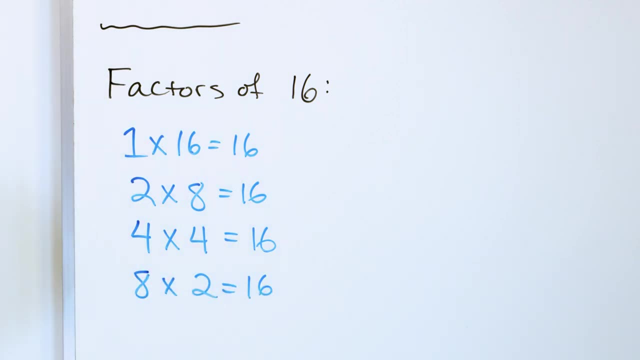 Then you go to eight, Eight times. Oh, I remember from my multiplication tables that eight times two is also equal to 16.. Eight times two is also equal to 16.. So those are factors. And then I go up to nine, ten, 11,, 12.. 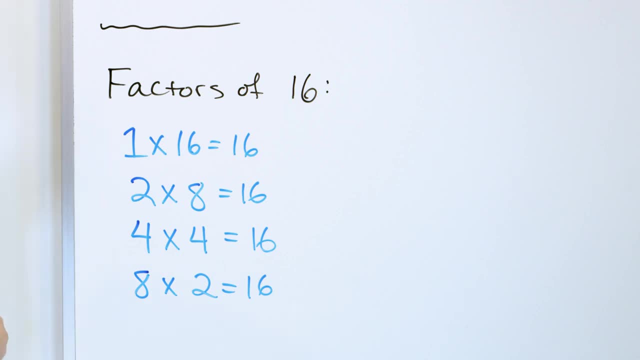 And eventually I just can't find any more numbers that multiply to give me 16.. So if I'm going to write the factors down, the factors of 16 are going to go like this: First we'll have the smallest factor, which is one. 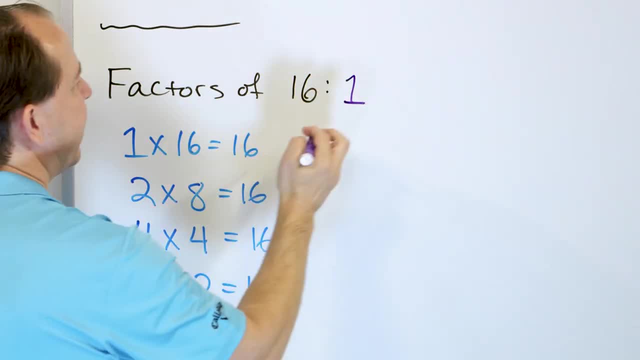 Then I'll write the factors in increasing order. Two is a factor And I keep going here. Four is a factor. Yes, I know that I have a four written two times, but I only pick the. I don't count duplicates. 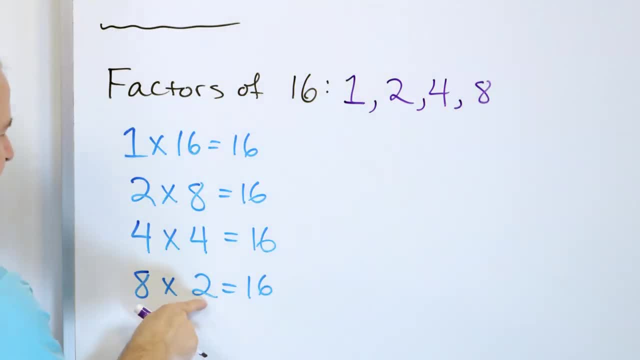 And then I see that eight is a factor, And again see I have a two here, but I already wrote two as a factor from a four, so I don't write it again. So it's one, then two, then four, then eight. 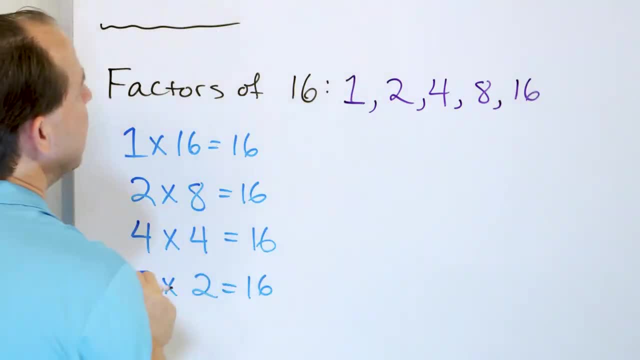 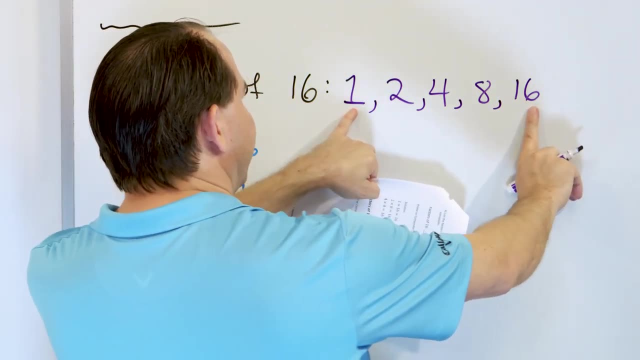 And that looks like that's all that there is. So then there's 16, of course That's a factor. So you see, factors of 16 always has a factor of the number one and always has the number itself as a factor. 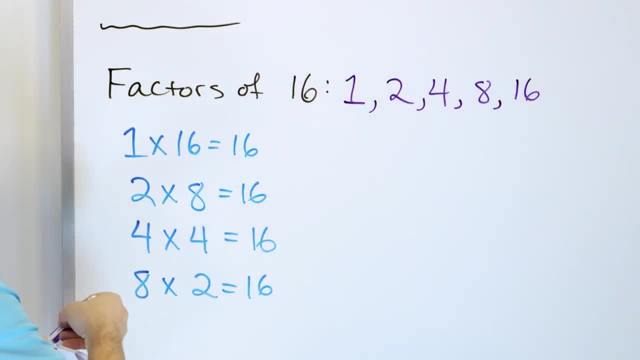 These numbers in the middle are the additional factors: The two, the four and the eight. those are also factors because they can multiply to give 16.. Two times eight is 16.. Four times four is 16, and so on, right. 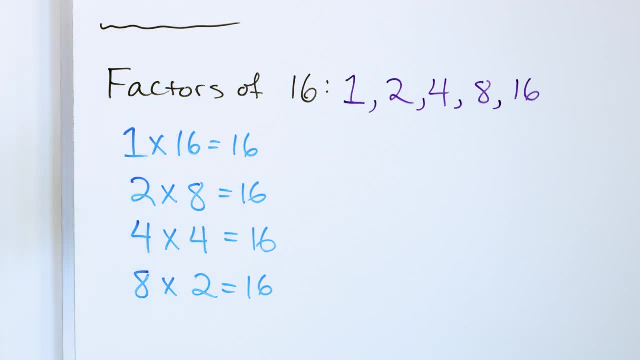 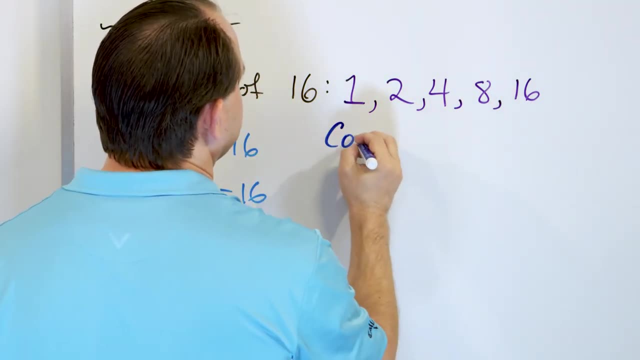 So is this number a prime number or a composite number? Remember, prime number only has the factors, that are the number itself and the number one. This thing has tons of factors, so it's a composite number. It's a composite number. 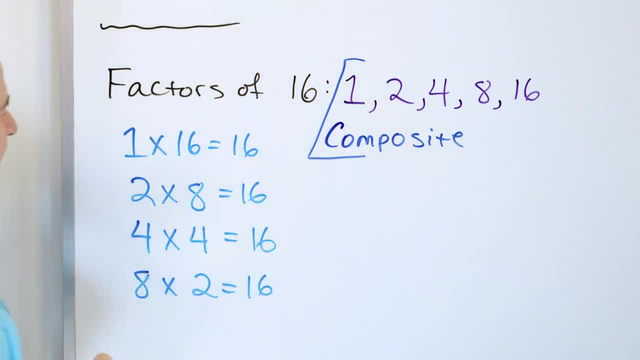 So what we will do is circle all of that, because I want to list the factors of the number and I also want to list if it's prime or composite. Now you see, let's go off and write our factor tree here. 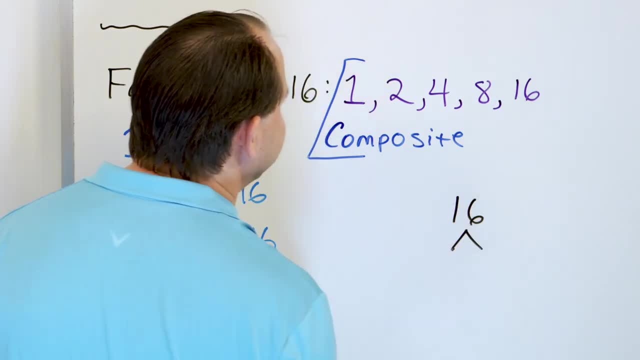 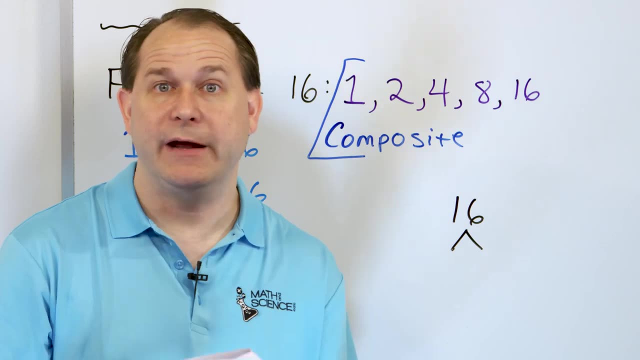 We're going to write the number 16, and we're going to try to use it to predict the same factors here, because it gets a little bit. You see how long it would take if I gave you, you know, 59 or 58 or something. 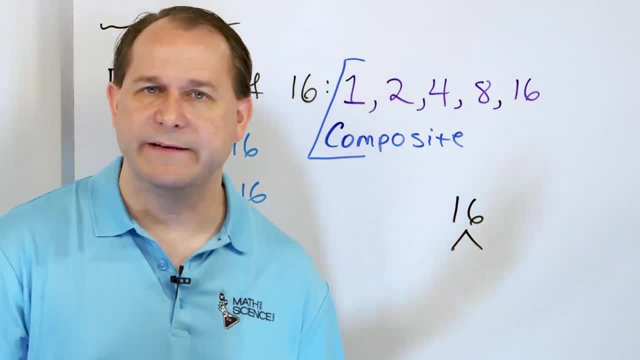 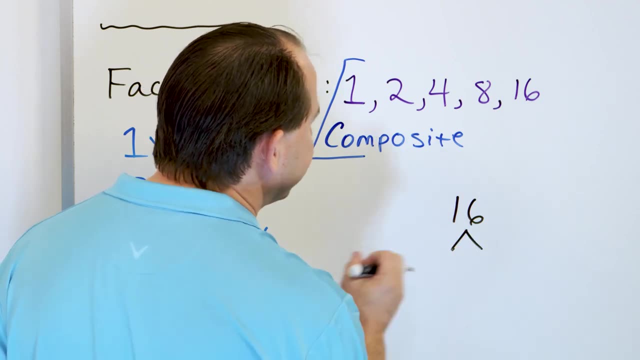 and said: tell me the factors. You'd be thinking about it forever, writing all these things down. So let's look at it like this: When I get to this, I can build this factor tree any way I want. Let me first build it with anything times anything. 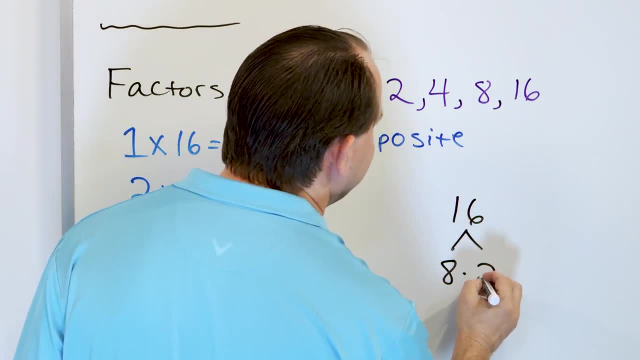 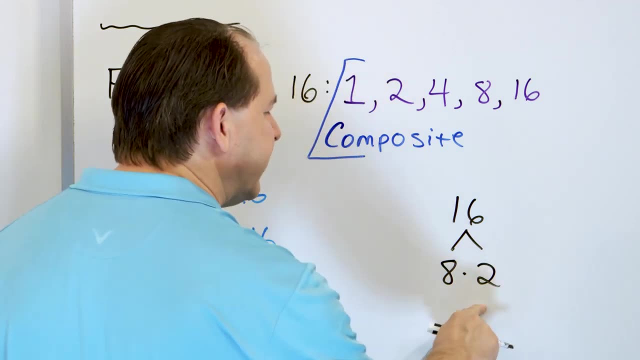 to give me 16.. So let's think about eight times two. Eight times two is 16.. I know that that's true. Now I can't really break the two any further, because two is prime right. Only one times two is two. 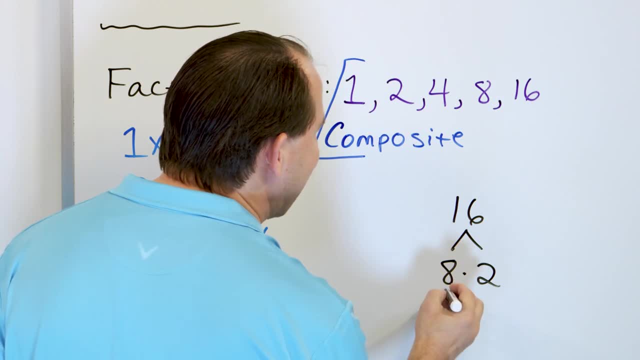 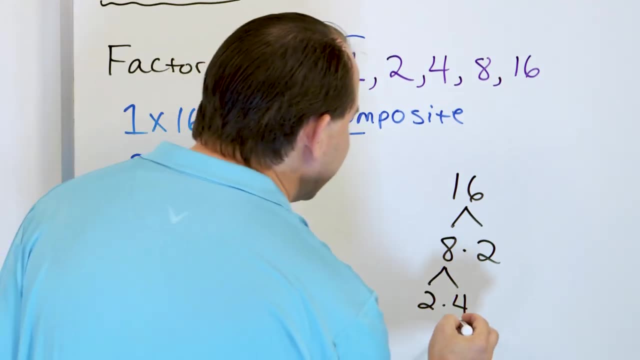 so I don't need to go any further there. But eight, of course I can break eight down further. Eight I can write as two times four. Two times four, right, And this four I can write it as two times two. 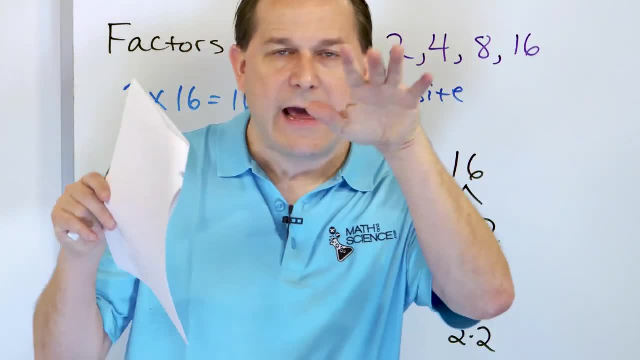 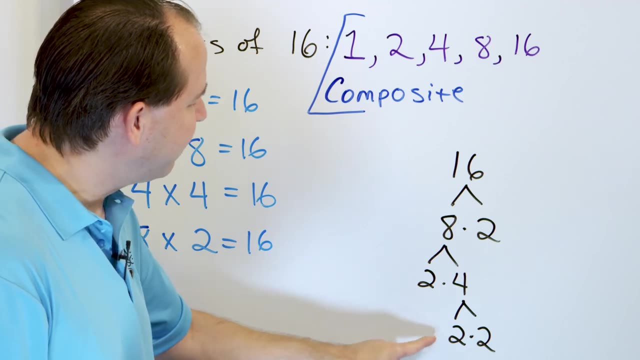 So you see, what I'm doing is I'm just going down the tree and I'm breaking every number that I have into the smallest numbers that multiply Now, of course, two. you can go as one times two. Two can go as one times two. 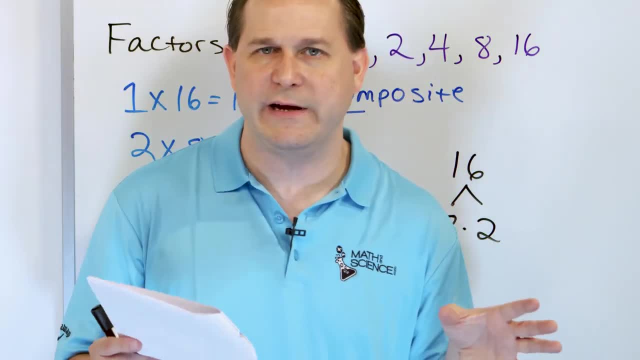 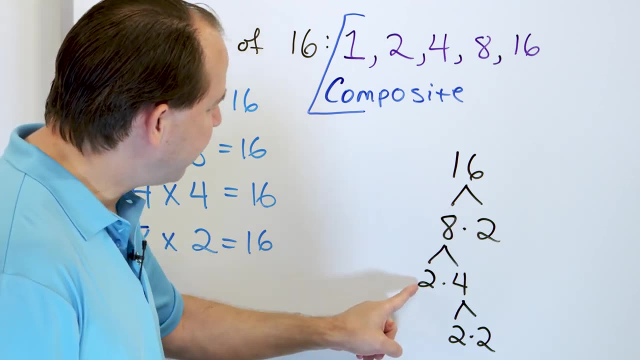 but when you get down to the point where the numbers at the bottom of the tree are just one times the number, then you don't really write them anymore. But 16 is eight times two, and then eight can be written as two times four. 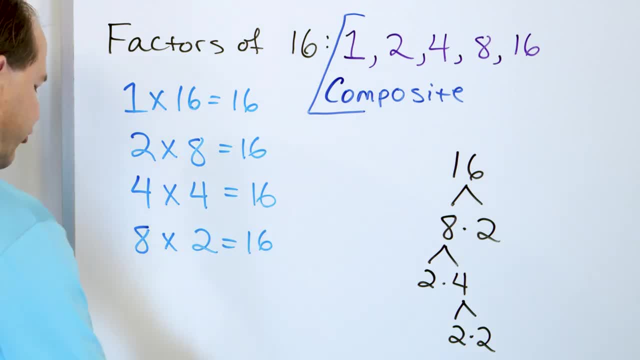 and then four can be written as two times two and I stop And then I'm going to try to read these factors, the additional factors off the tree. So if I'm trying to write the factors of 16, I know that one is a factor. 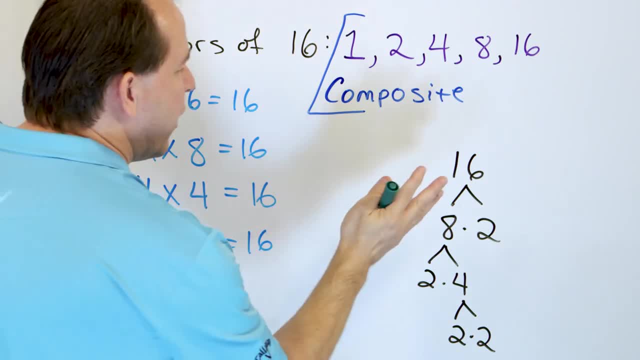 I know that 16 is a factor, so I write those down. But on the tree I immediately see that two is a factor because it's at the bottom of the tree, so that has to go in there. I see that four is a factor. 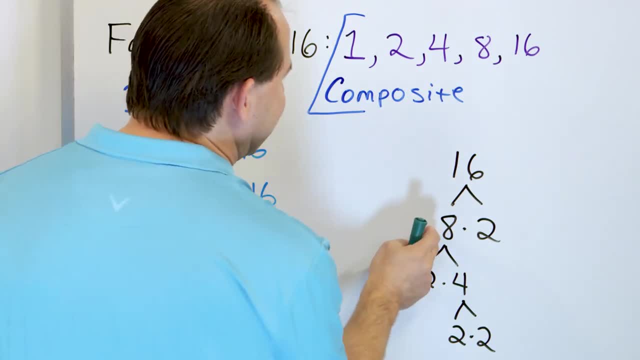 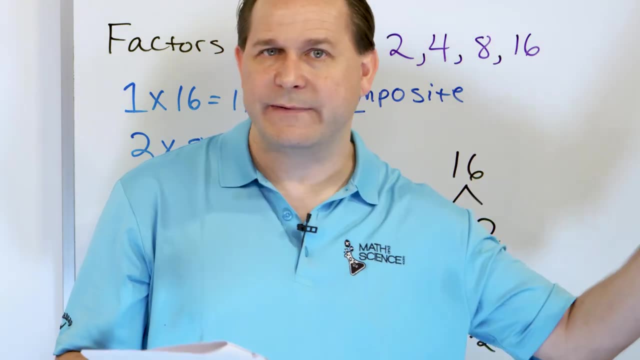 so that goes in there. And I see that eight is a factor, so that goes in there. So basically, any numbers that you see in the tree, any numbers you see in the tree at all, you write them down as factors because it's called a factor tree. 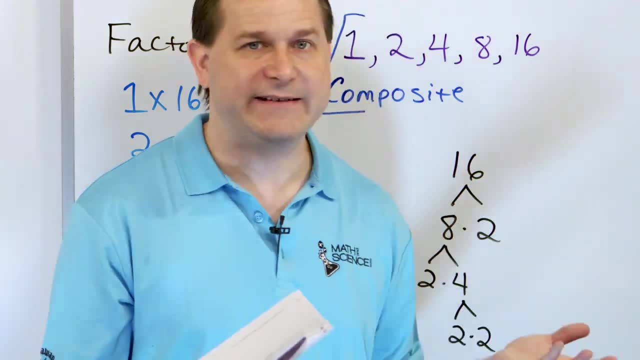 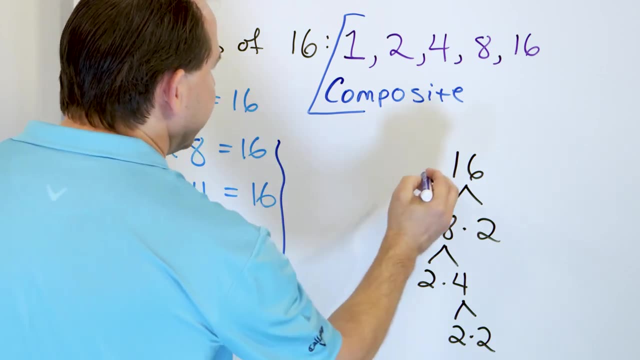 You're writing things down that multiply together to give you, in this case, 16.. So any of these numbers are factors. Now I want to show you really quickly what would happen if you chose a slightly different tree. Let's do the exact same thing. 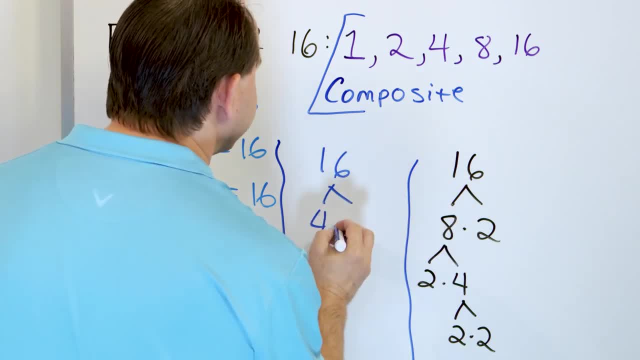 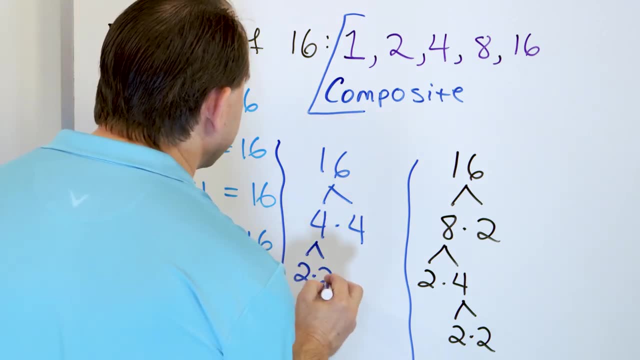 16.. Instead of 18, let's say you did four times four, because that also makes 16, right, Okay? So then you say here's four times four, All right. So this is two times two And this is two times two. 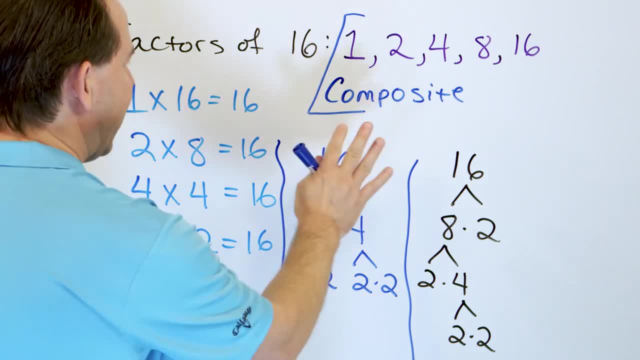 Remember the dots just mean multiplication. So I look, Let's say I don't even have this as a factor tree. I want to use this factor tree to figure out the factors. So what do I do? I say all right. 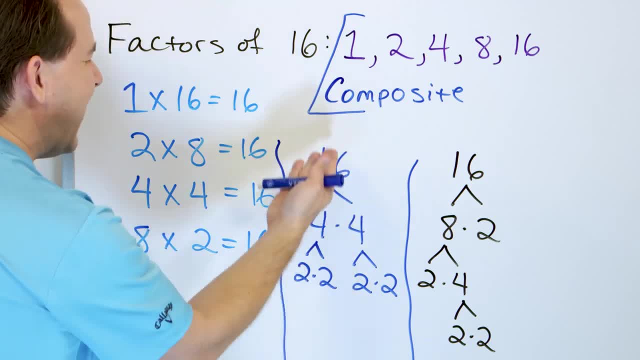 two is a factor, I put it in there. Four is a factor, I put it in there, But there's no eight in this tree. So I'm like, what do I do? There's no eight in that. How do I find all the factors? 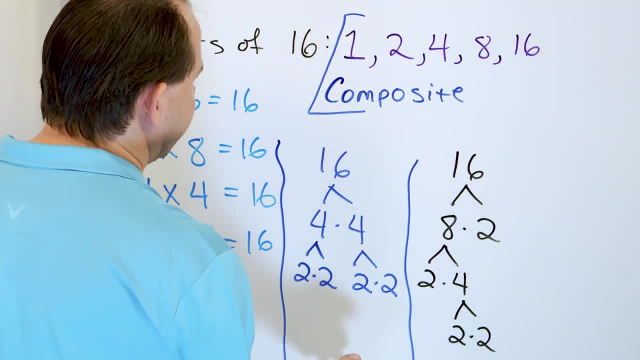 So here's what you do When you build your factor tree: all the numbers that are written there you put in your list of factors, But also any numbers in this branch of the tree over here and any numbers in this branch over here. 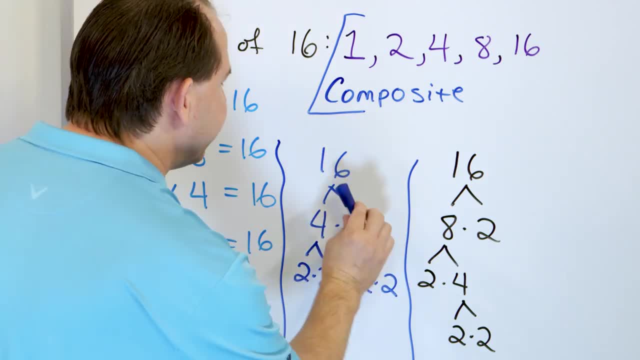 you can multiply branch to branch and it gives you even more factors. So you see, I have a four here and I have a two in this branch, So I can multiply four times two and that gives me eight, and that's a factor right. 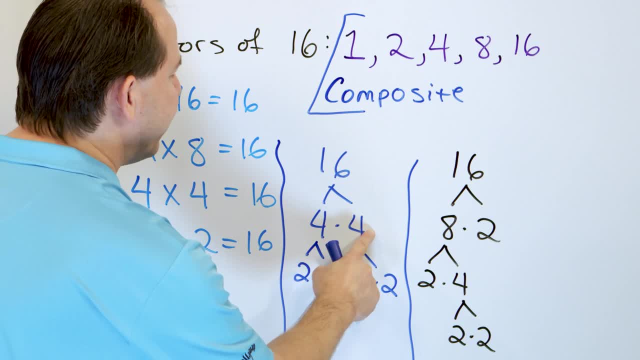 Of course, this four times this two is eight. It's a duplicate. So what I guess, what I'm trying to do is I'm going to multiply four times two and that gives me eight, and that's a factor, right, Of course. 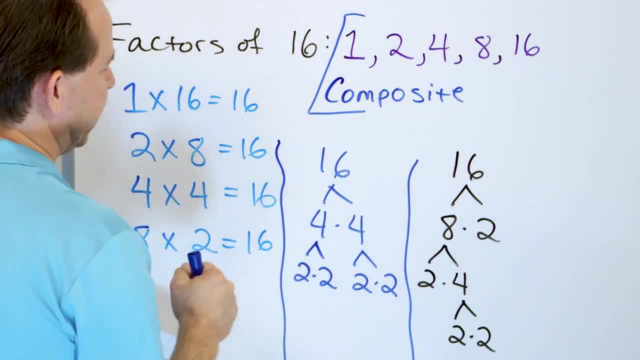 this four times, this two is eight. It's a duplicate. So what? I guess what I'm trying to say is: build your factor tree- and I'm going to show you lots of practice with it- and you write down all the factors that are in the tree. 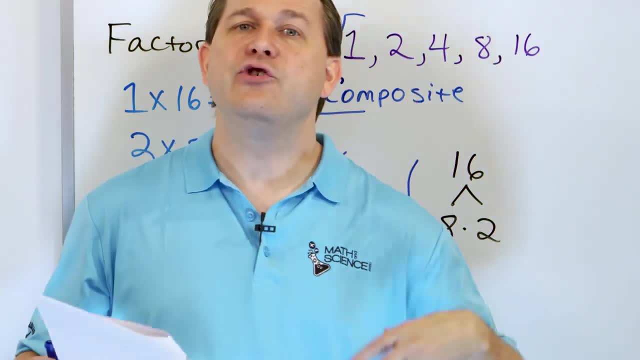 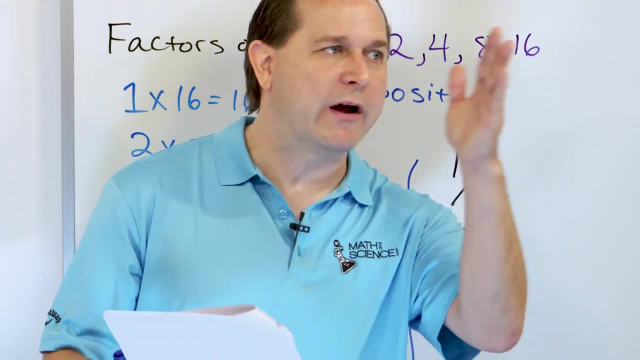 But then you also cross-multiply the branches here to here, here to here, looking for any more factors. Any other numbers you get by cross-multiplying the branches are also factors. You might say: well, it was much easier just listing them out. 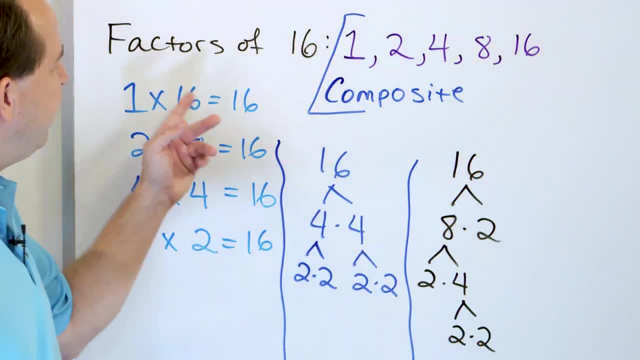 I agree with you For the number 16, it's easier. But when I give you the number 96, it's going to be a factor. So what I'm trying to do is I'm going to show you all the factors. 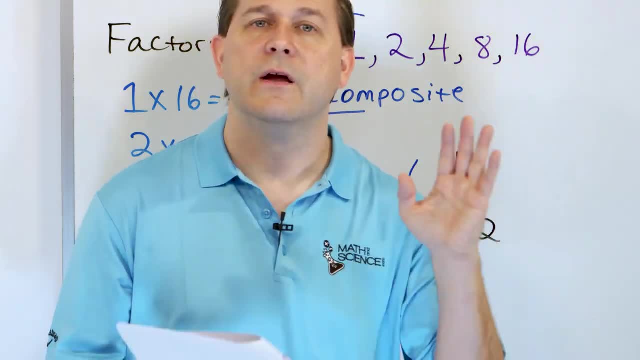 that are in the tree. And then when I give you the number 86, it's going to be harder to think of all those things that multiply. So we're going to be using factor trees there. So no matter what tree you pick. 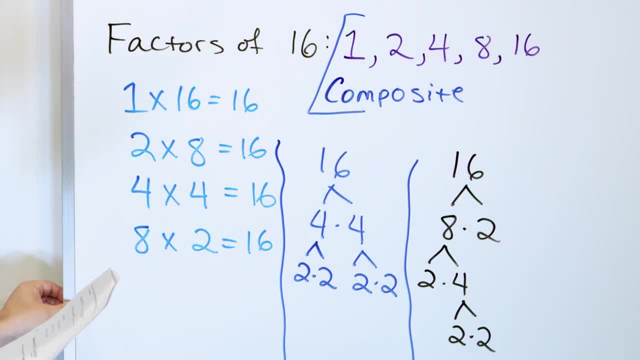 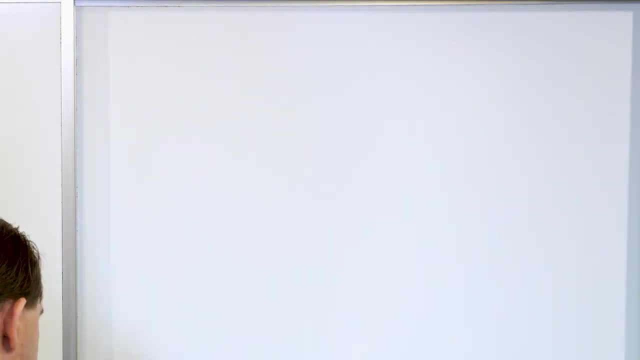 what you actually end up doing on your paper. you will end up at all of the factors there And of course, it's a composite number. All right. Next we have to. I think we have two more problems We want to list. 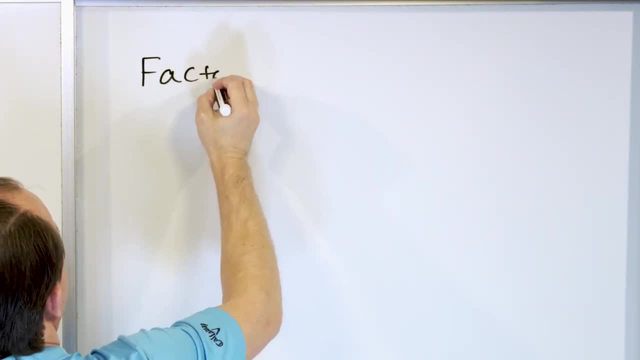 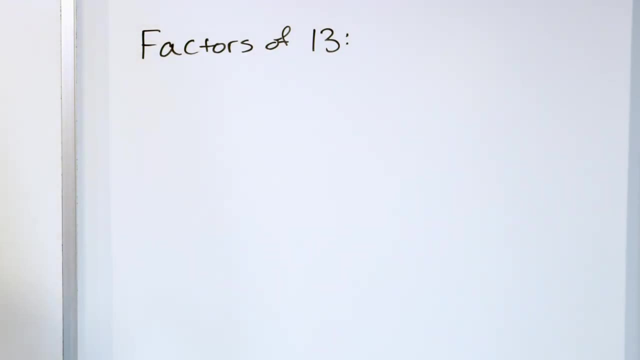 the factors, of want to list the factors of 13.. All right, So we start thinking through it. What times? what is 13?? Well, I remember, of course, 1 times 13 is 13.. Right, And then what is? 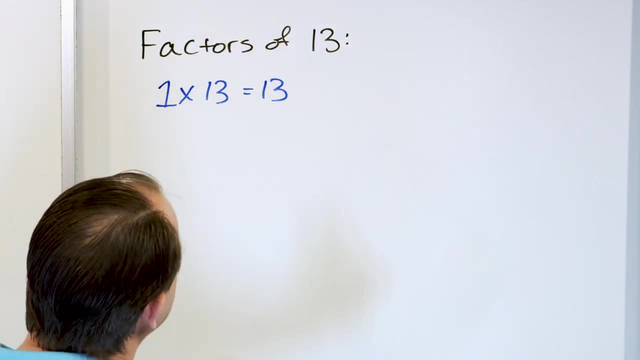 2 times something is 13?. 3 times something is 13.. 4 times something is 13.. It doesn't look like anything else. times anything can give me 13.. So the factors are just 1 and 13.. 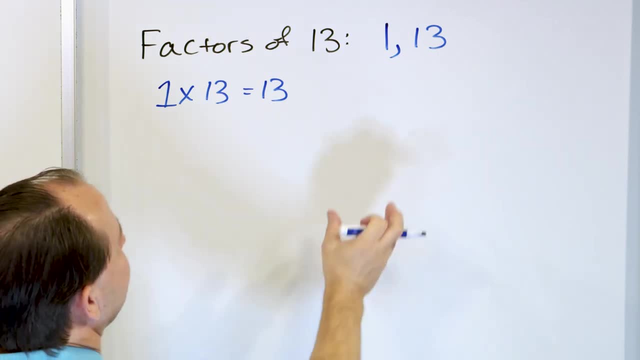 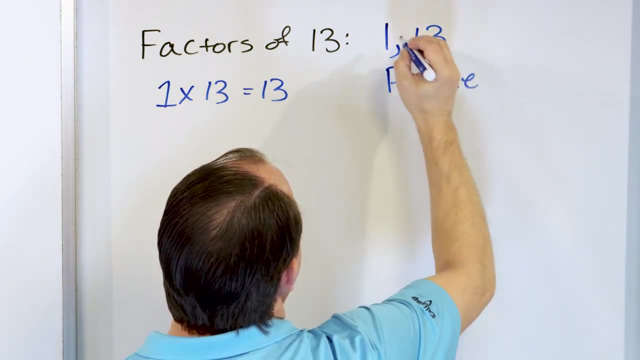 That's what I think the answer is, And because there's only two factors, the number itself and the number 1, this thing is called prime. It's a prime number. 13 is a prime number. So what we say is: 13 is a prime number. 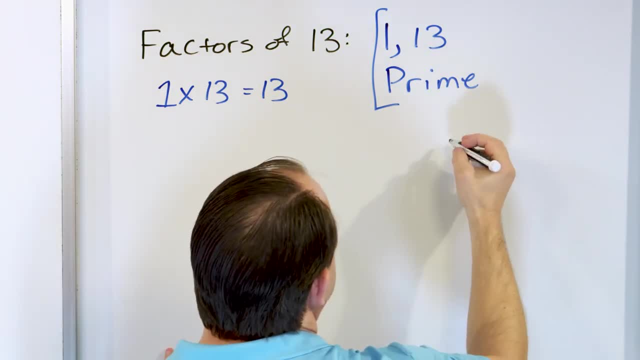 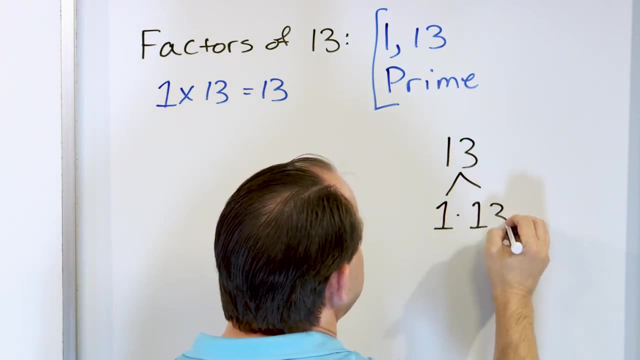 And then, of course, we can try to do our factor tree. We'll put the word, the number 13.. Think of: anything times anything is 13.. The only thing I can come up with is 1 times 13.. And then I have. 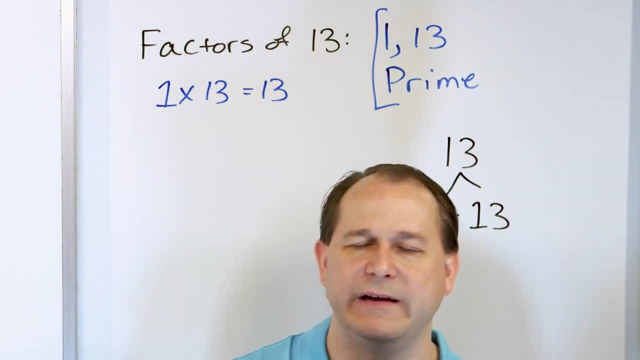 a 13 here, but I can't break that any further because, again, the only thing I can think of is 1 times 13.. So the factor tree tells me the only factors are 1 and 13,, which means it's a prime number. 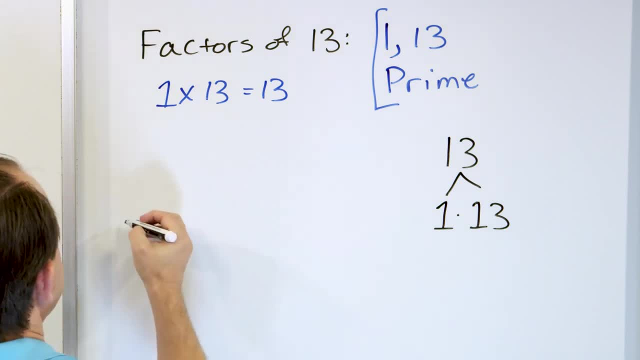 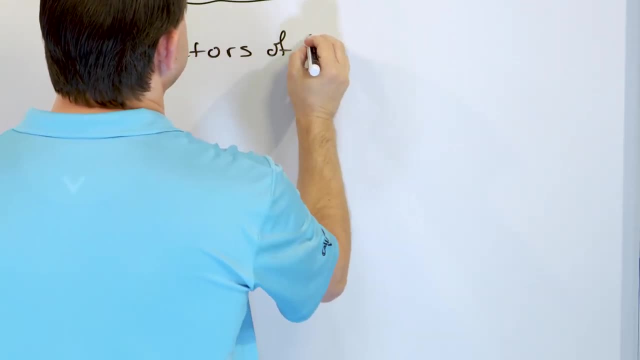 All right, I think we have. I was wrong. Let's take a look at the next problem. Let's take a look at the factors of the number 7.. So we just go through our multiplication tables. We say, well, we know that. 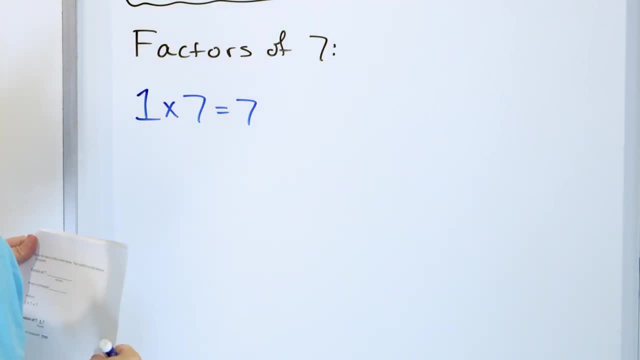 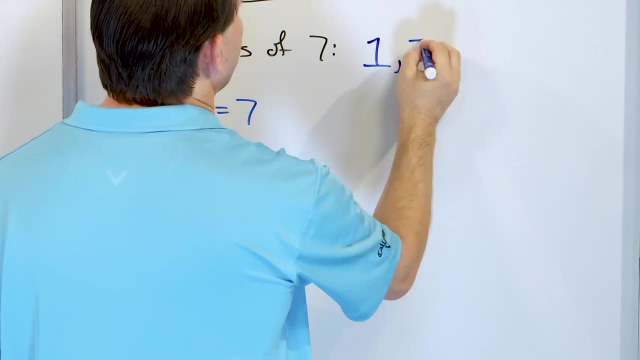 1 times 7 is 7., 2 times. oh, I can't think of anything as 7.. 3 times 3 times something, 4 times something, 5 times something, 6 times something. I can't think. 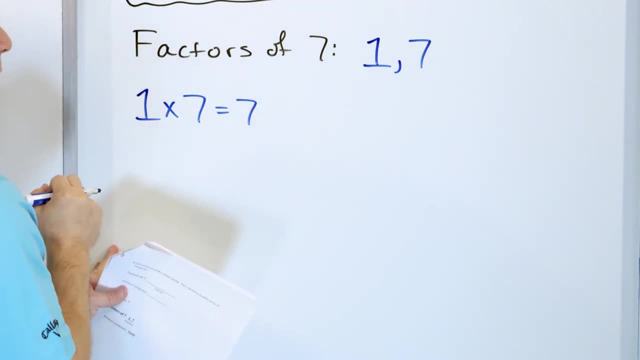 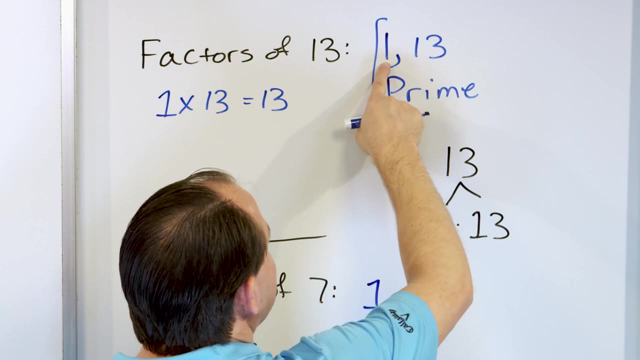 of anything else. So the only numbers are 1 and 7 that I can think of that multiply to give me 7, and 7 times 1 is 7.. So it goes in the list, Just like 1 times 13.. 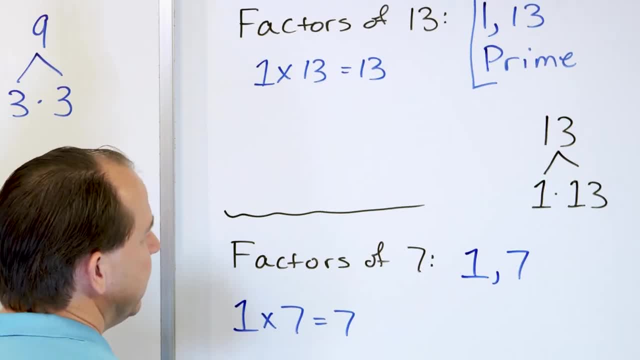 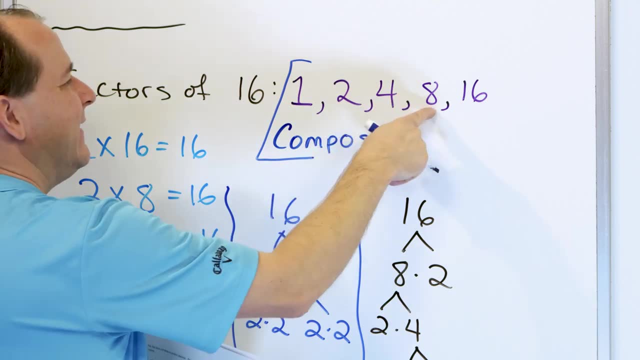 So 1 goes in the list and 13 times 1.. So 13 goes in the list. All right, When I go over here, I know that 1 times 16 is 16.. 2 times 8 is 16.. 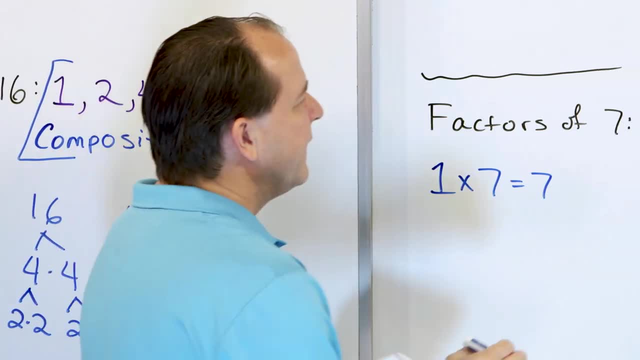 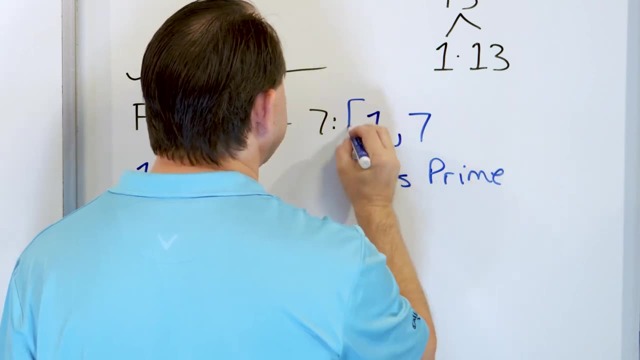 4 times 4 is 16.. 8 times 2 is 16.. 16 times 1 is 16.. So all of them go in the list, But this one only has 2.. So we say that the number 7 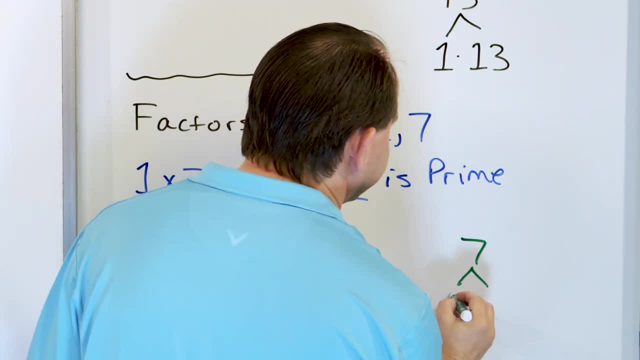 is prime. We don't really need 2 for this one, But all you would do is you would do 7 times 1.. And I can't break them out any further. There's nothing else there, So there's only 2 factors. 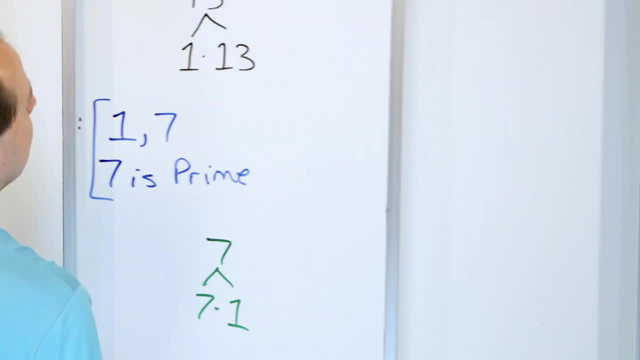 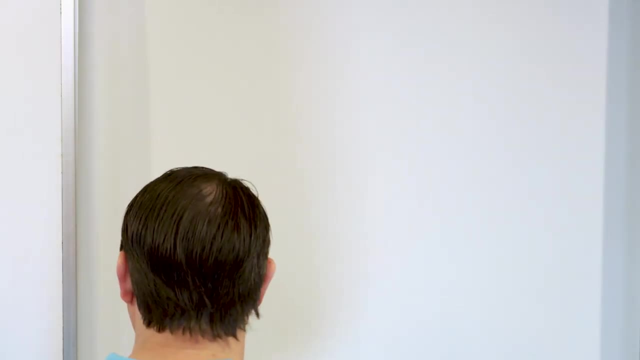 and that's all you have to say is that 7 is prime, because there's only these 2 factors. That's it All right. So let's go back to a larger number that you're going to be using a lot in math. 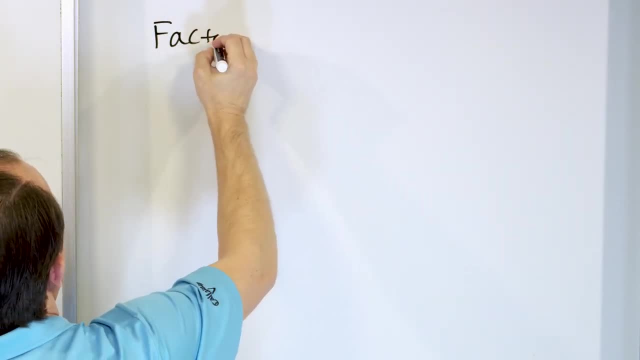 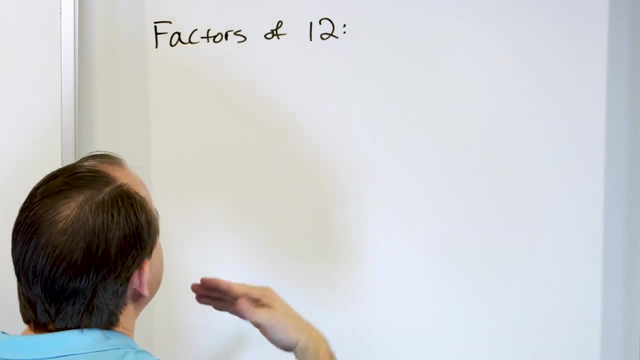 The number 12 comes up all the time. Let's find the factors of 12.. Let's find the factors of 12.. All right, So we're going to do it in a slightly different way. Let's just go through our multiplication. 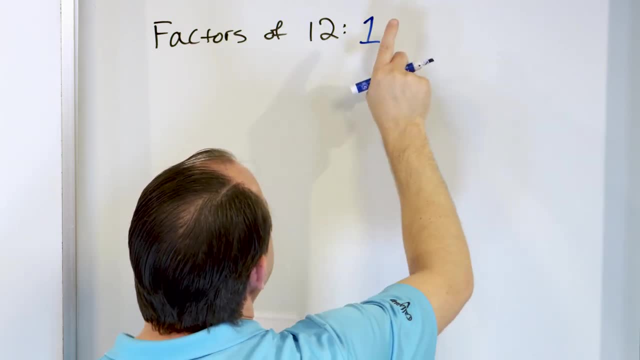 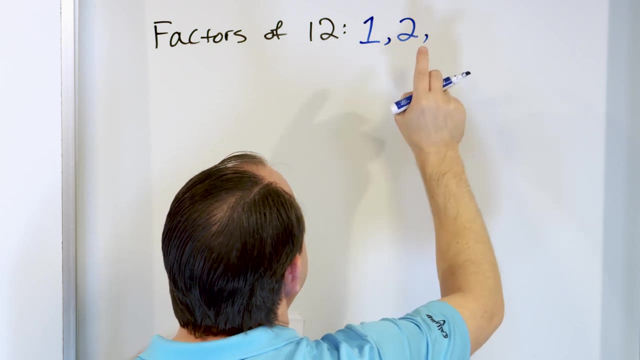 tables. Let's just try to write the factors down. We know that 1 times 12 is 12.. So 1 is a factor, Then we go up to 2.. We know that 2 times 6 is 12.. 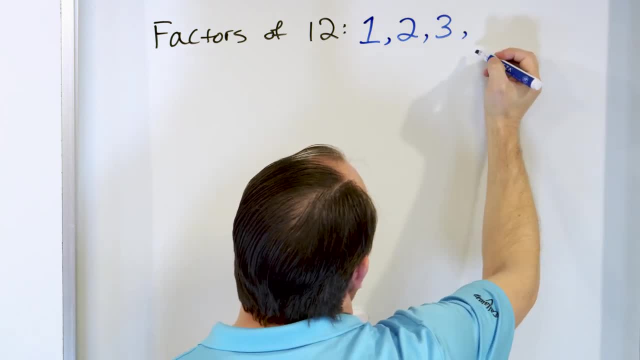 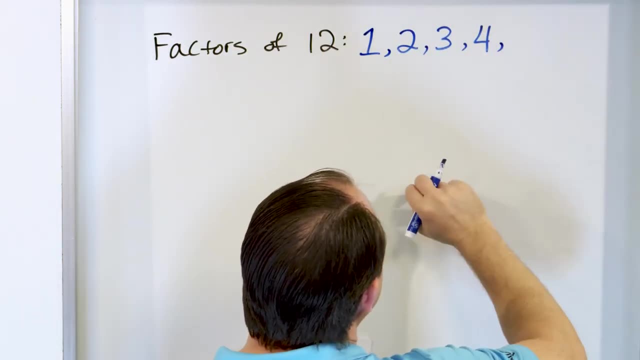 So 2 is also a factor, All right, 3.. Let's think about it: 3 times something is 12.. 3 times 4 is 12.. So 3 is a factor 6 times. oh, 6 times 2. 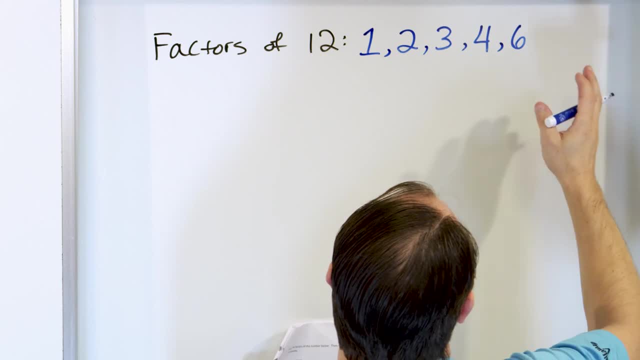 is 12.. So that's a factor: 7 times something, 8 times something, 9 times something, 10 times something, 11 times something. None of those make 12.. But then we get finally to 12.. 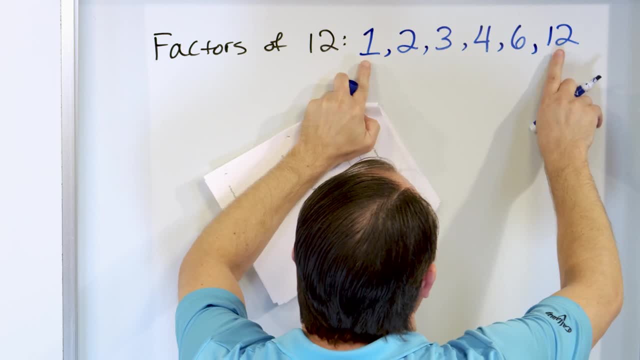 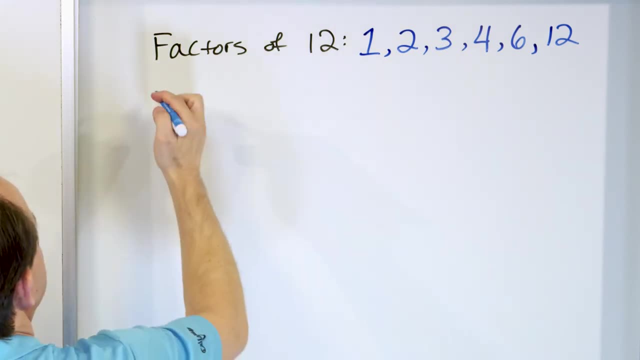 12 times 1 is 12.. So you see, you always have the two factors that are like the core factors: 1 times 12 is 12.. The rest of these come from your multiplication tables And I'll just 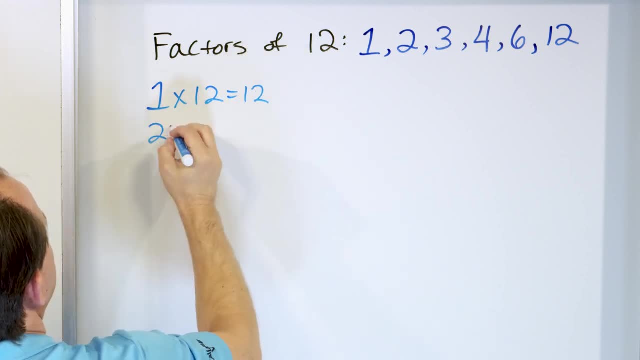 you know, be 100% clear, We know that 1 times 12 is 12.. We know that 3 times 4 is 12.. So basically, we can get all the factors by writing down what multiplies 12.. 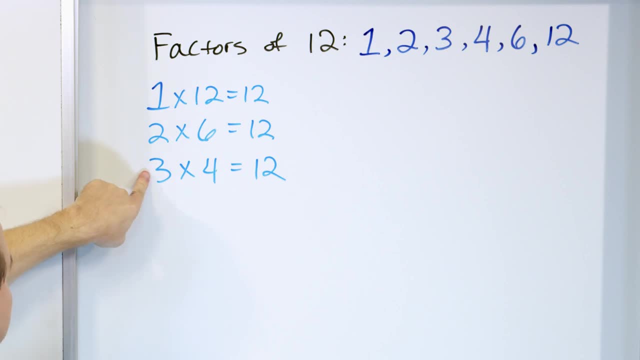 1 is a factor, Then 2 is a factor, Then 3 is a factor, 4 is a factor And then 6 is a factor And 12 is a factor. I've just listed all the factors here, All right. 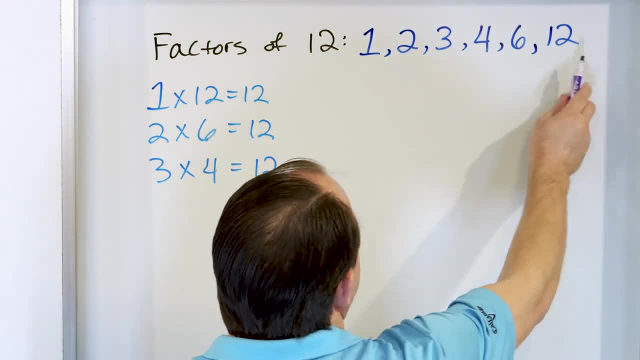 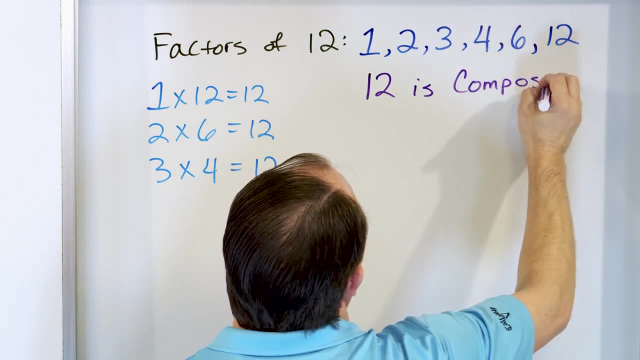 So how many factors do we have? We have a ton of them. Is this prime or composite? We know now that 12 is composite. Basically, if it has more than two factors, you know, then it's going to be a composite number. 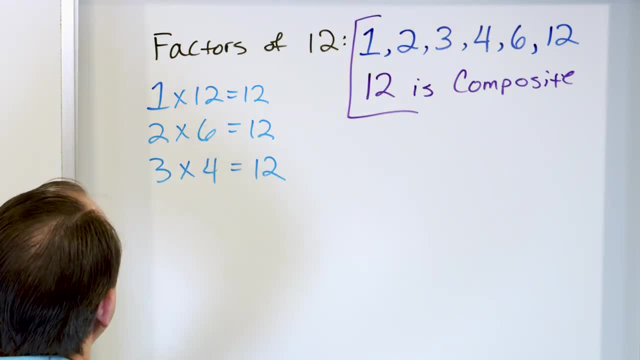 So we circle that. That's our answer. Now the last thing I want to do is go ahead and try it with the factor tree. Let's put the 12 here And we're going to build this factor tree and see if we can recover. 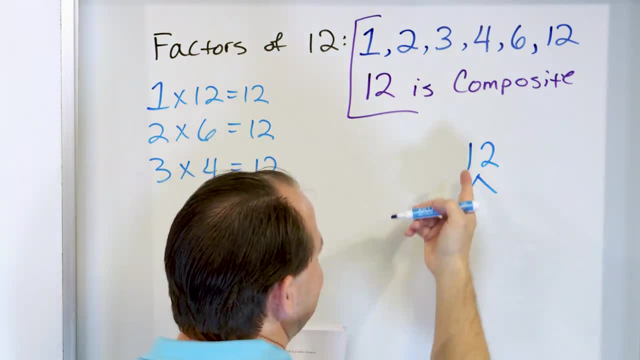 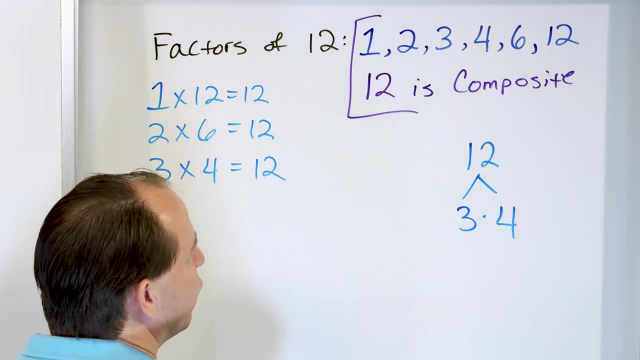 all the factors, because when we get to larger numbers, we're going to primarily use the tree here, So you can do whatever you want. The first thing that pops in my mind is 3 times 4. That's 12.. Now I can't really. 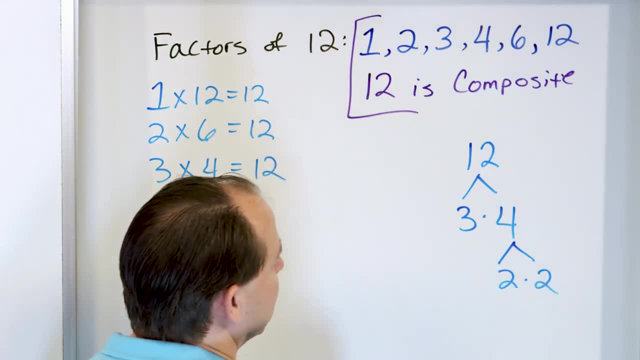 break out 3, because the only thing I want to do is write out that 2 times 2 is 4.. Now I can't really break the 4s out, the 2s out anymore, because only 1 times 2. 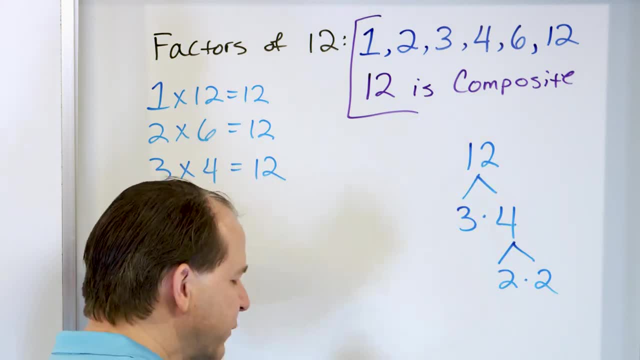 is 2.. So I don't need to write anything more, But this is a complete tree for the number 12. 3 times 4 and then 2 times 2.. Now again, I could do the tree a different way. 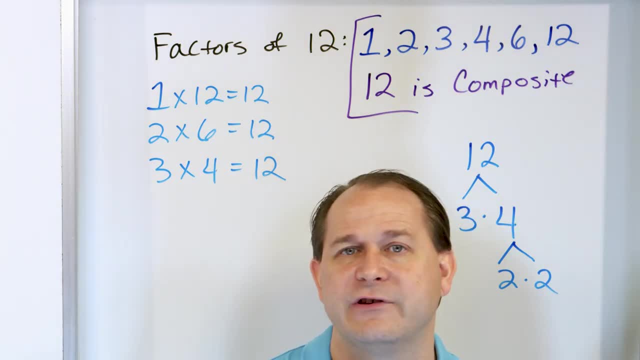 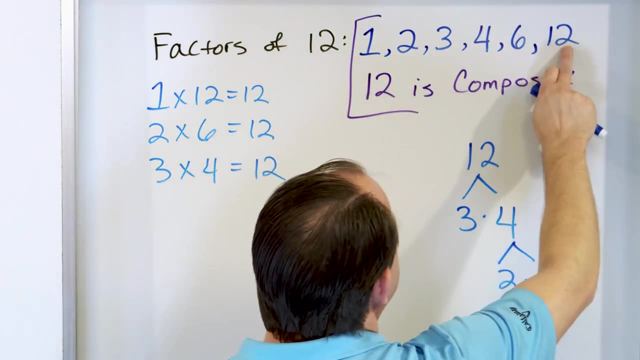 Instead of 3 times 4,, I could have picked: 6 times 2 is 12. And it would be a slightly different looking tree, but it would get the same information out of it. So let's just use what we have here. 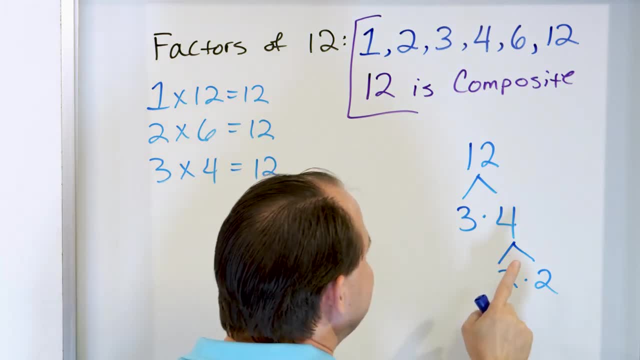 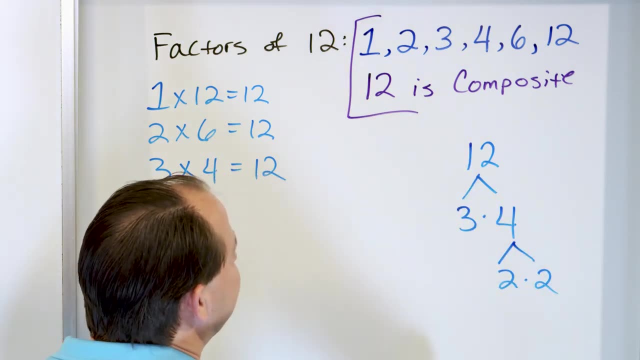 What we want to do is figure out from the tree anything extra. So we can see that 2 is a factor, We can see that 3 is a factor And we can see 4 is a factor. We read them all out of the tree. 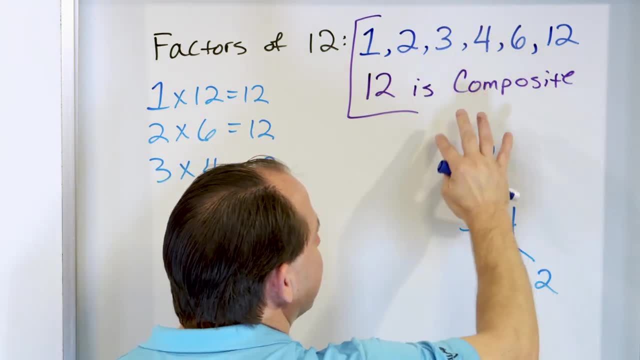 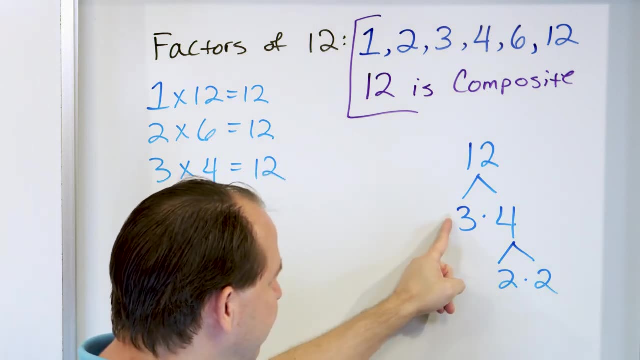 Any number you see in this tree is a factor: 2,, 3, and 4.. Right, But look at this: The number 6, we know is a factor, but it's not in the tree. But I also told you extra factors. 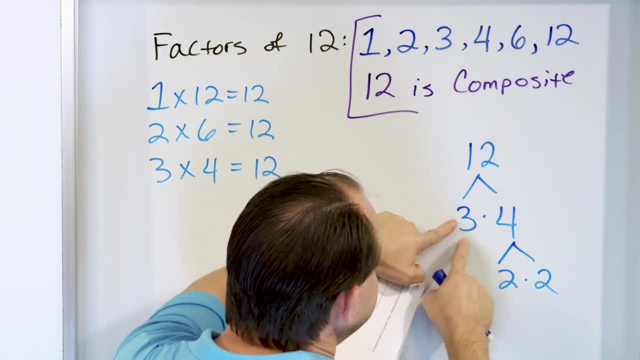 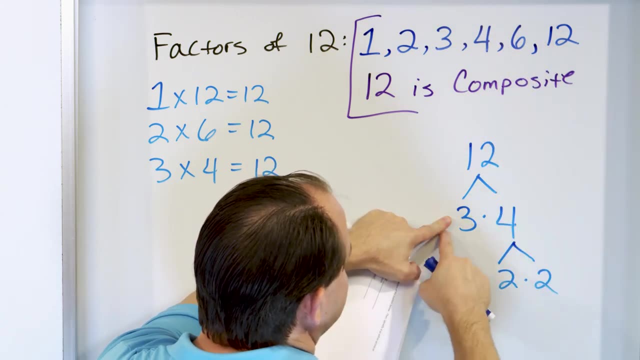 you can get, by multiplying the different branches, Any number in this branch times any number in this branch. So here we have 3 times 4, right, 3 times 4 is 12, but we already know 12 is a factor, so we can put that up. 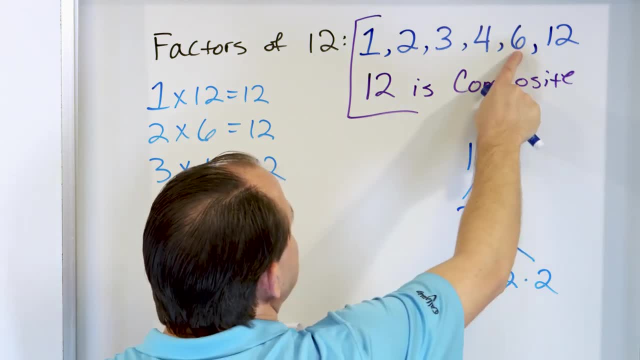 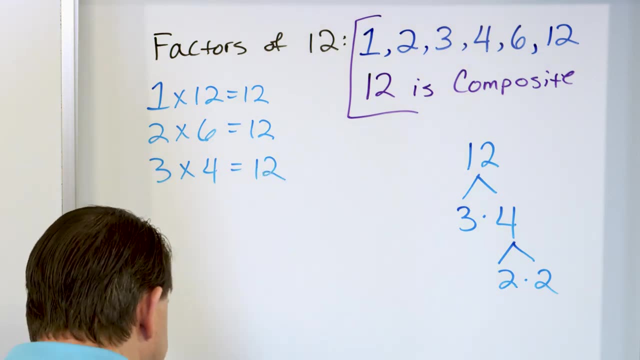 there as well. But we know we can get an extra factor by looking at 3 and multiplying by one of these 2. so 6 is a factor. and look at that. we already had it in our list, So the tree can be used. 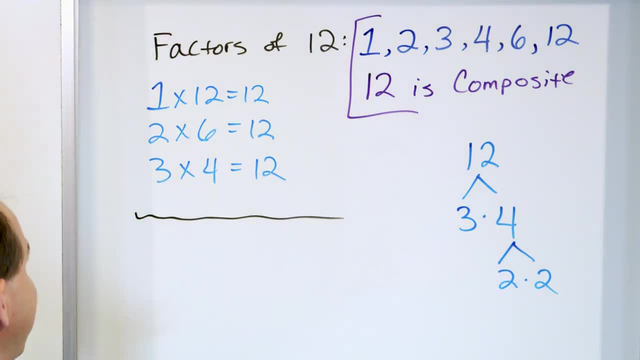 to give me all those extra factors. I'm trying to teach you for the small numbers because for the big numbers it's going to really save us actually a lot of time. So the factors are 1,, 2,, 3,, 4,. 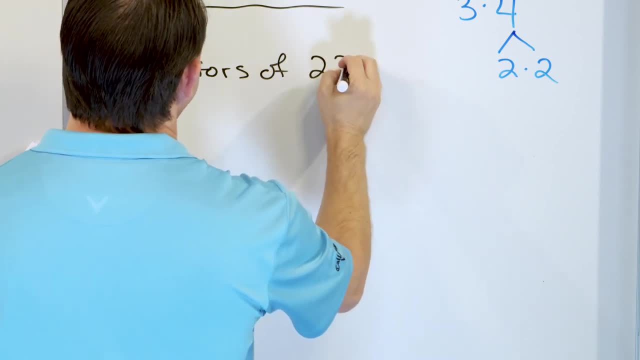 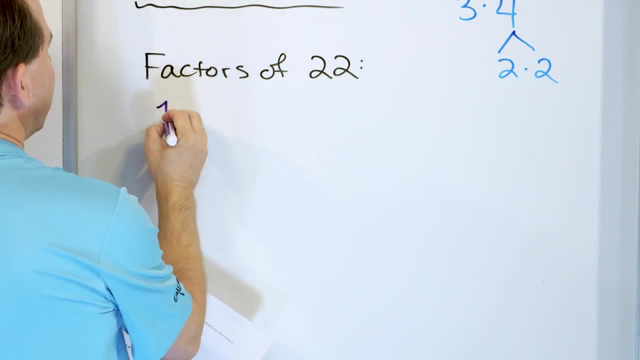 6, and 12 of the number 22.. The factors of the number 22.. Let's first just try to do it by thinking about the multiplication tables. Well, we always start with the number 1.. 1 times 22. 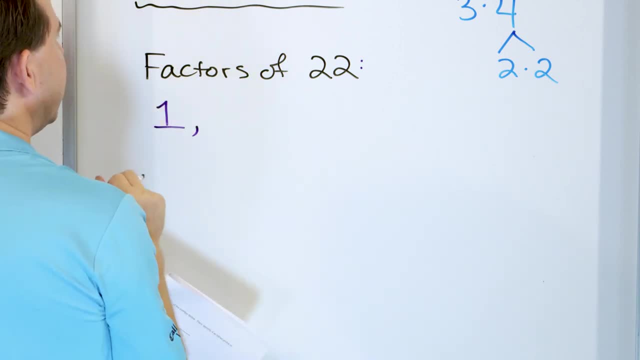 is 22. so we know that's right. We go to 2.. Okay, 2 times what is 22? 2 times 11. so we know that 2 is a factor. We go to 3 and 4 and 5. 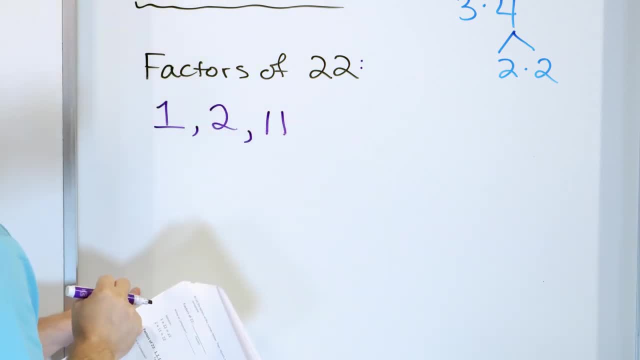 and we don't find anything else that multiplies to give us 22. but eventually we get to 11, so nothing else multiplies to give us 22 until we get to the number 22.. So we know that 1 times 22 is a factor. 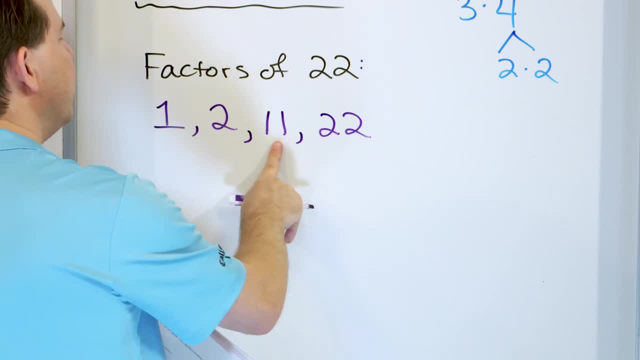 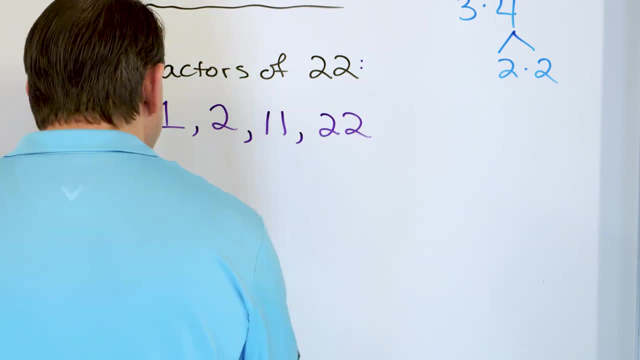 2 times. so 1 is a factor. 2 times 11 means 2 is a factor. 11 times 2 means 11 is a factor. 22 times 1 is there, so we know it's a factor. So 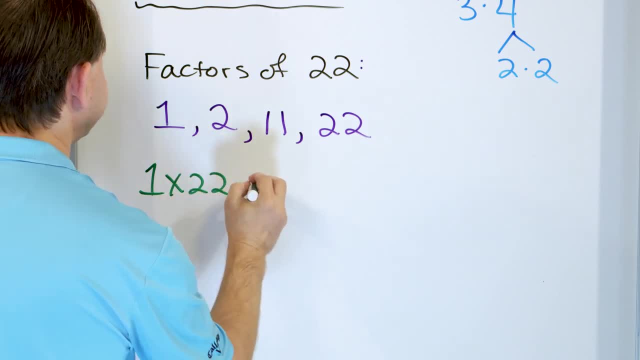 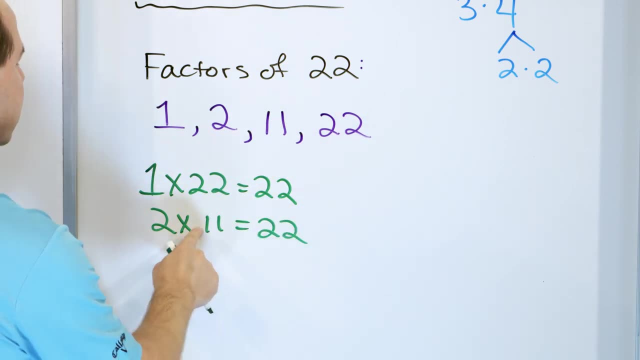 if you really want to multiply it, we know that 1 times 22 is 22.. We know that 2 times 11 is 22. so really, all the information is here: 11 is a factor and 22 is a factor Right now. 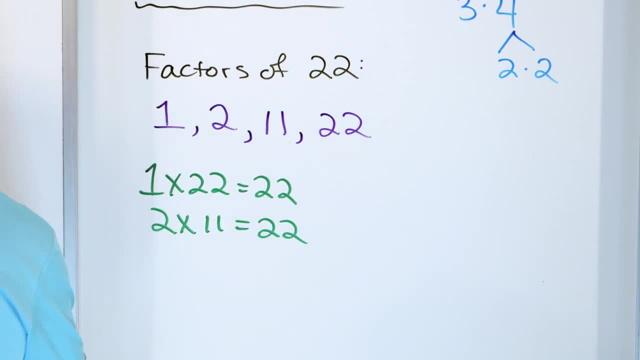 is this a prime or composite number? So we know from this that this is then a composite number, so I'll just write it. I guess I'll write it over here. I'll just write it right here: Composite, Composite number. Right Alright? 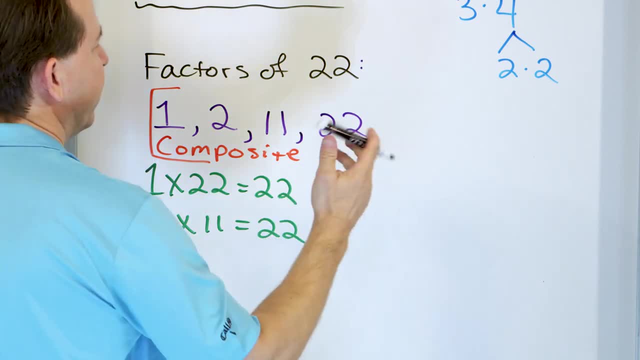 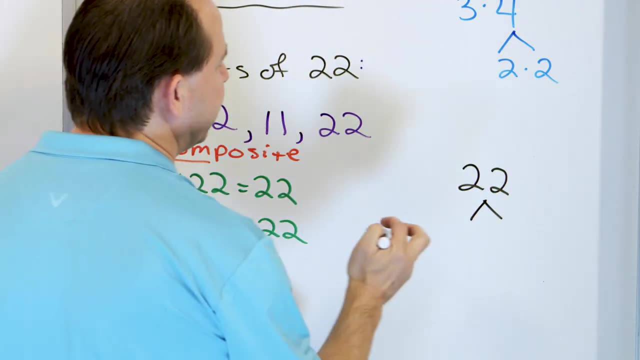 so then let's try it with our factor tree. We want to look at the number 22.. So you think you can pick anything you want, the first thing that pops in your mind that applies to give you 22.. For me it's 11 times 2.. 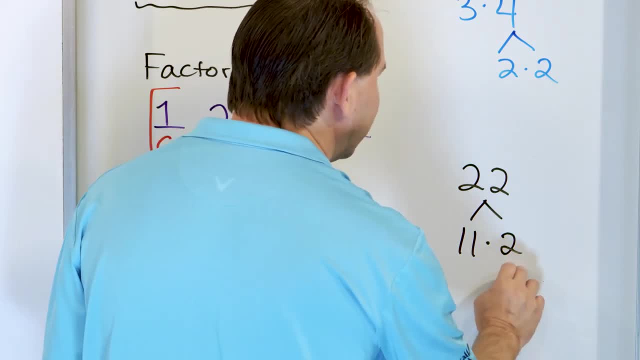 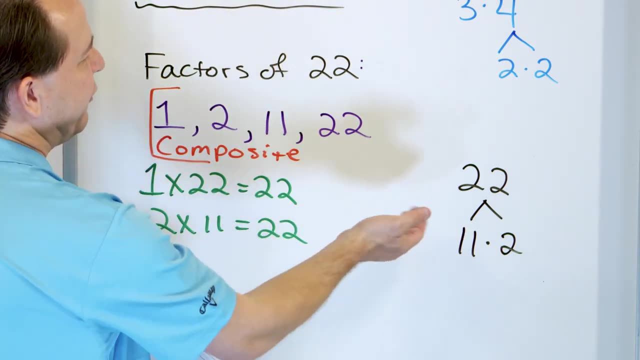 I know that's 22.. Then I try to break these down further. For 2, there's only 1 times 2, so I can't go any further. and for 11, the only thing that works is 11 times 1, so I can't really. 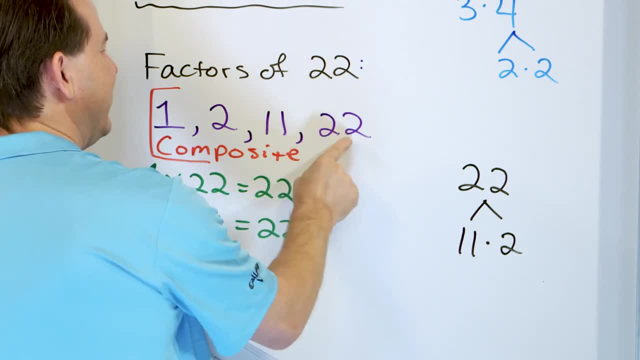 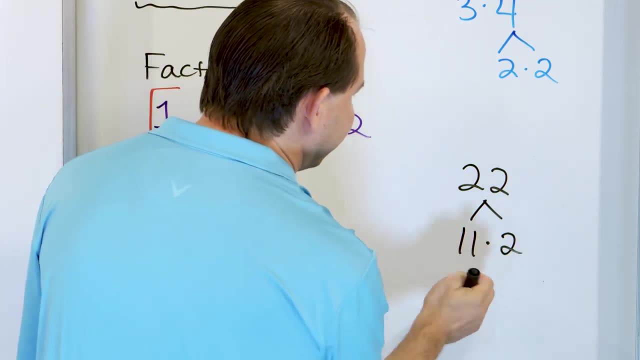 go further there. So my tree is done. So I know that the number 1 is a factor and I know that the number itself, 22, is a factor. so I look in the tree for other ones. I see that 2 and 11.